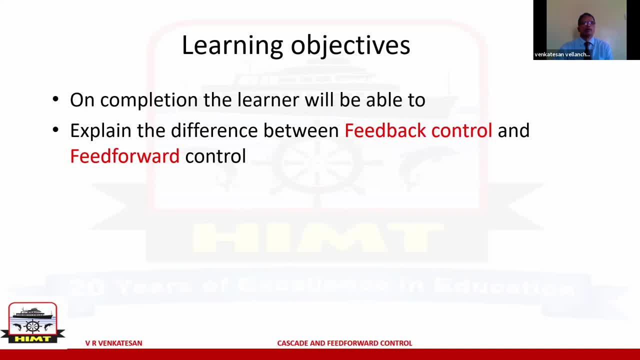 control and feed forward control. There will be examples of applications of feed forward control. We will see examples where feedback and feed forward are both used together. We will see examples of cascade control. To recap what we have already covered so far in the previous lectures. 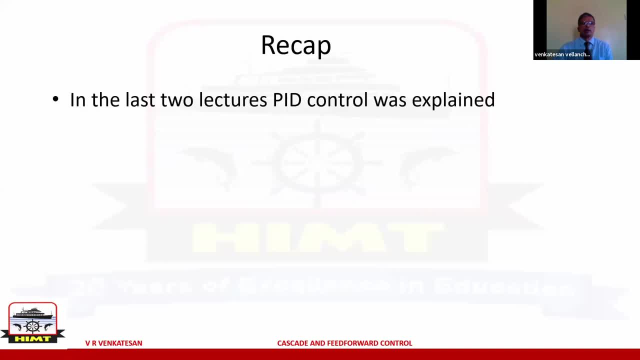 in the last two lectures I'd mentioned that PID control was covered: Proportional, Integral and Derivative control and combinations Proportional plus Integral and Proportional plus Derivative. So to look at it quickly, Proportional control is the basic control action. 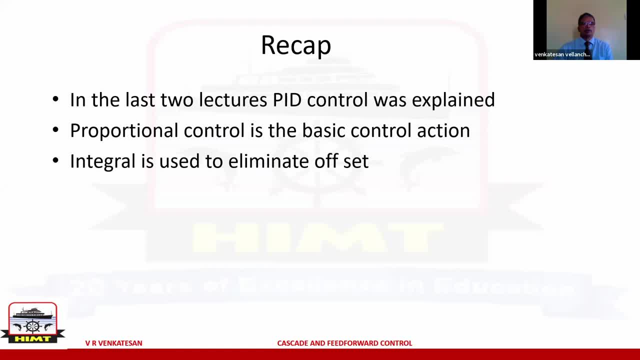 Integral control is used to eliminate offset, and Derivative control gives quick correction without venting. This is the basic understanding of these three control actions, And P plus I is the most common type of process control application. as a general rule, around 70-75% of process controllers uses P plus I And only another 20% will require Derivative. 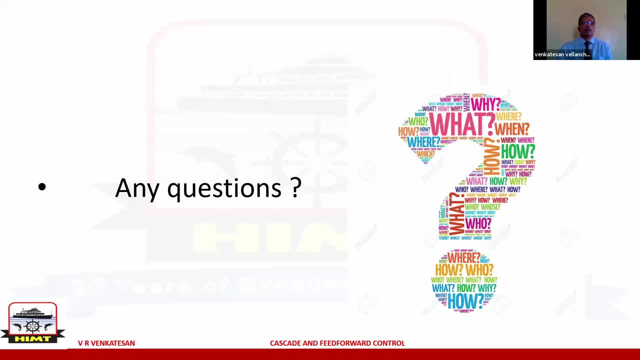 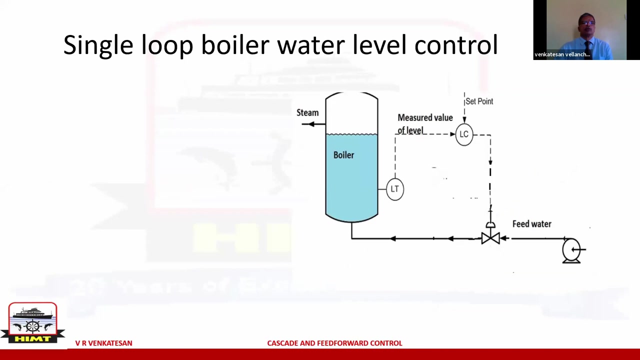 Are there any questions from the previous lectures? before we move on, No questions in the chat. sir, You can go ahead. Okay, fine. So what we are looking at is an example of boiler water level control. It is called a single loop boiler water level control. 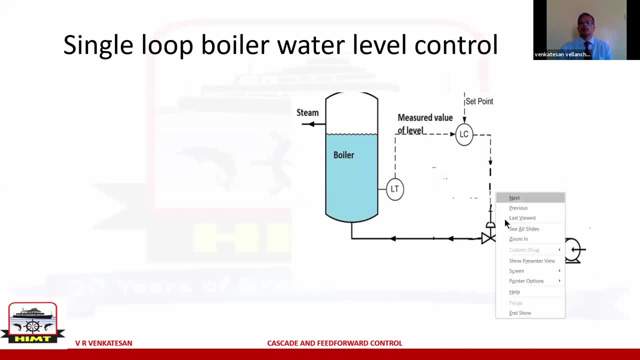 From the picture you can make out, there is a level transmitter. From the level transmitter, the measured value of level goes to a level controller. To this level controller, the set point is given. This is the set point. So this is measured value and this is the. 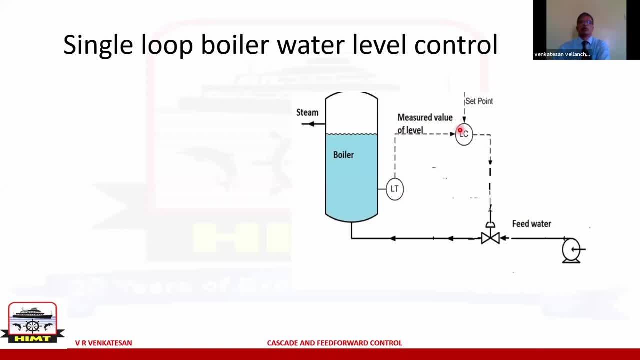 desired value. What will be the difference between these two, called different between measured and desired value, Error signal Deviation, Error signal Deviation, Or you can call it deviation. So the deviation is acted on and you will turn it into an output. 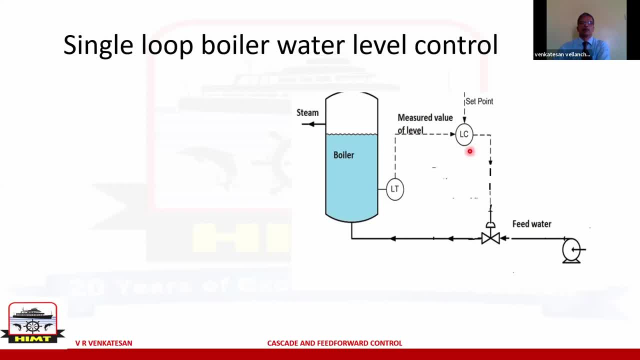 Boiler level control most commonly is P plus I, Unless it is for a propulsion boiler, in which case PID may be required. For auxiliary boilers purposes, P plus I is sufficient. So this level controller generates an output and it goes to the fuel. 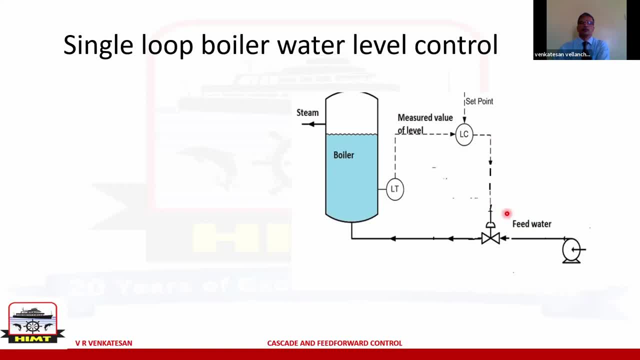 So this is a very common application. The way this will work is steam flow changes, For example. if the steam flow will increase, the water level will fall down And the drop in water level is detected and it is compared against the actual water level is compared. 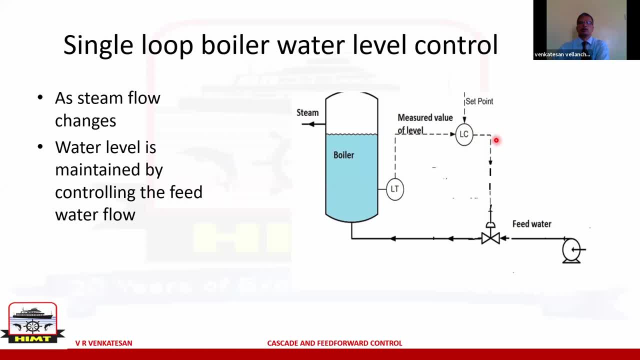 against the set point, Deviation is produced. Deviation becomes an output. So this is a very common application And the feed valve is open or closed. The output of the level controller goes to the feed valve. This is the simple application. 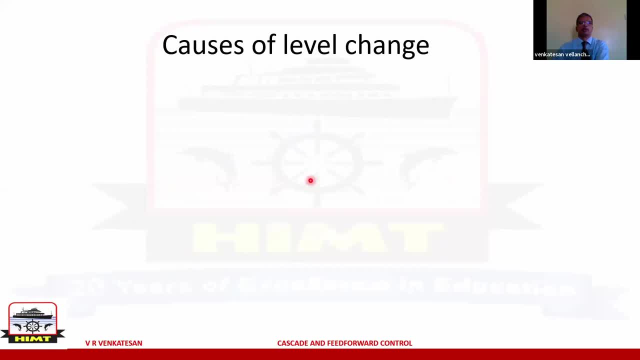 Very commonly used, But it has got some drawbacks. you will see What are the reasons level changes. Number one is steam demand will change. It is the most common reason. After the steam demand changes, level will change. It will decrease, It will increase. 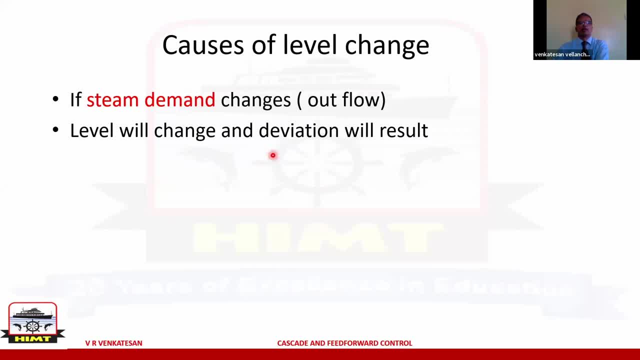 It will increase, It will decrease, And only after the level changes this controller can react. So it is not possible to avoid change in level. Only after level change takes place the correction can take place. You can also have a problem with the feed water inflow. 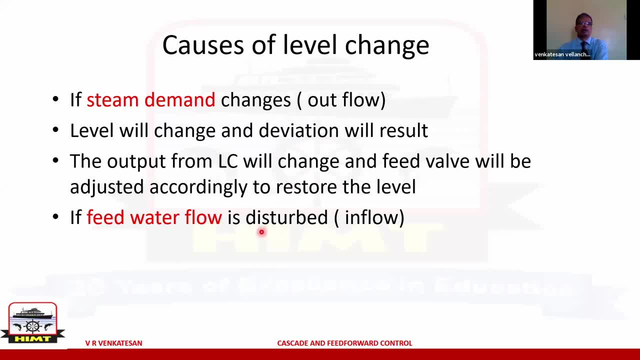 That water flowing into the boiler is less or more. In this case also, the level will change and control action will follow. So the controller is capable of facing or handling difficulties due to change in steam demand or change in feed water flow, But in either case level will change and only then the correction can take place. 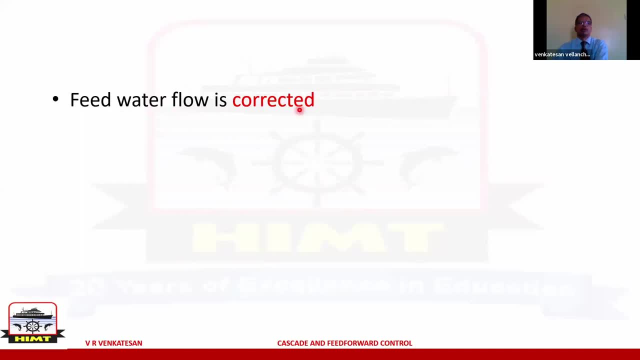 So what is corrected is feed water flow is corrected. Corrected is the level. What do you mean by corrected variable is the one which needs to be adjusted. Controlled variable is: what do you want to maintain? So, in the case of boiler water level, controlled variable is water level. corrected variable is the feed water flow. 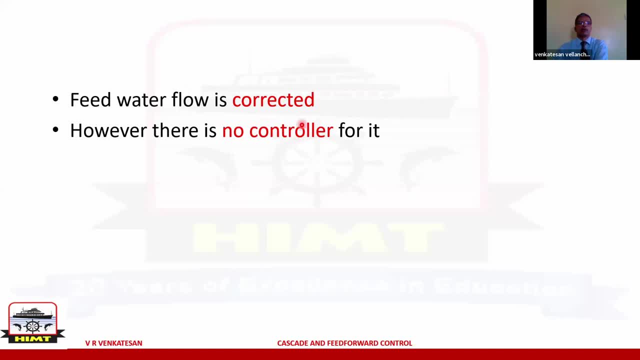 But there is no separate controller for the feed water flow itself. The controller is only for the level. So if you have issues, for example the feed valve does not move freely, The feed valve sticks, Then the correction will be delayed. 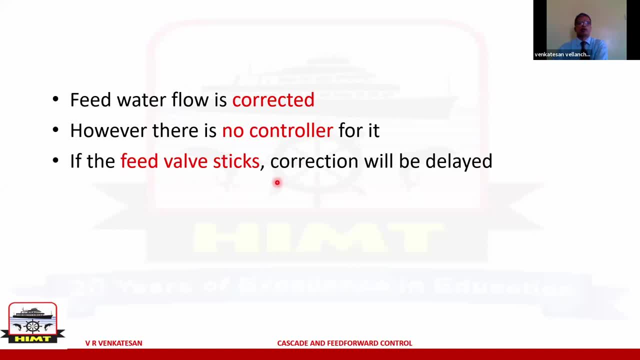 In the sense that water level will correct slowly, Deviation will build up And, if you remember, if you put integral control, what will be the result? Can anyone answer? No offset, Yeah, that is what you will get finally, But if the error persists, what will be the result? 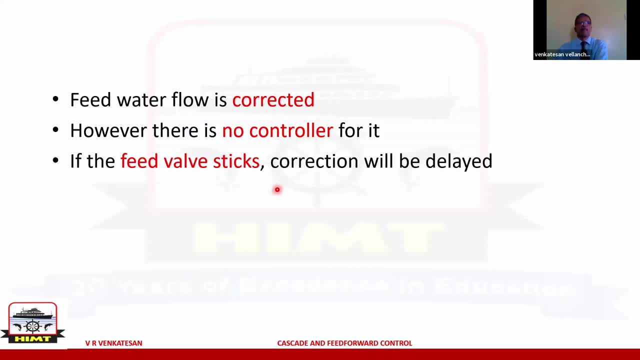 Integral control Output increases. Output will keep increasing, So the controller will take care of this problem by increasing the output and the feed valve will be opened more, But definitely there will be delay in this. One more problem is like when valve opens. 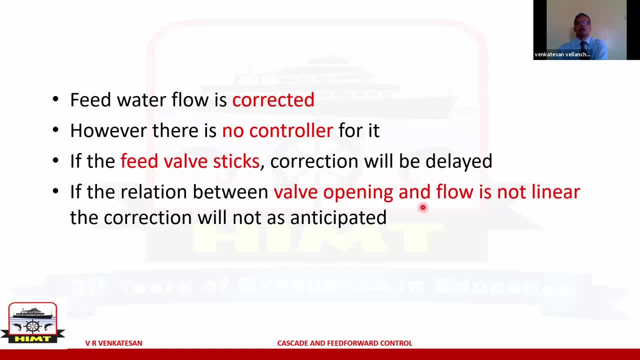 and the flow changes. this relation need not be linear. What does it mean? you have a linear relation. X is equal to constant Y, Right. Practically what this means is, if the valve opening increases by 20%, then the feed water flow also should increase by 20%. 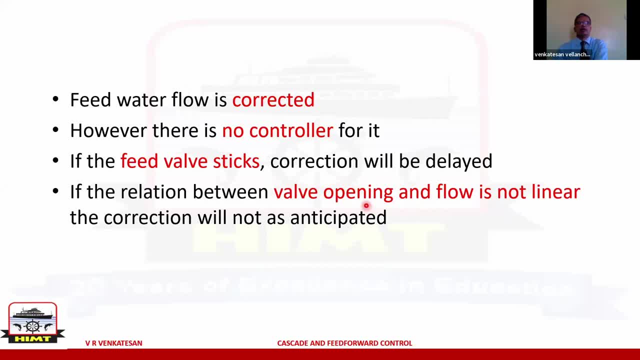 That is called linear relation. So if the relation is not linear, then also you will have difficulties in in control. Often the valves are chosen for linear relation, But if it is not correctly chosen or if there are any errors, then also the correction will not be as you expect. 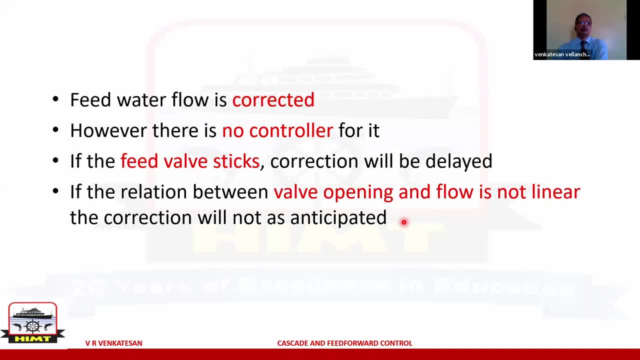 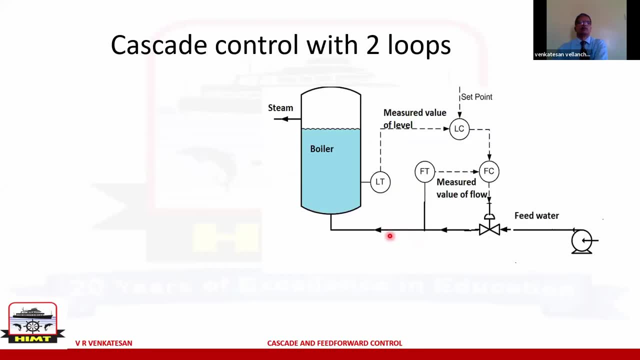 More errors will build up. So how can we tackle these kind of problems? What are the ways we can tackle? There is one method. This is called as cascade control. Cascade control is also called as master-slave control Control. What is the English meaning of the word cascade? 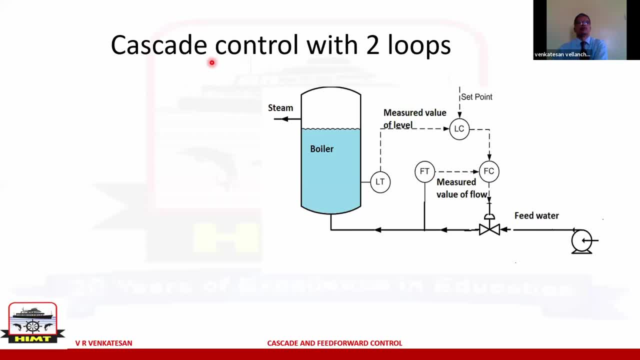 Never use the word cascade. What is it? Joining two different? Sorry, Not in control. In common English, what does cascade mean? Cascade actually means Fountain or waterfall. Waterfall, Exactly, Waterfall, which is Which drops in steps. 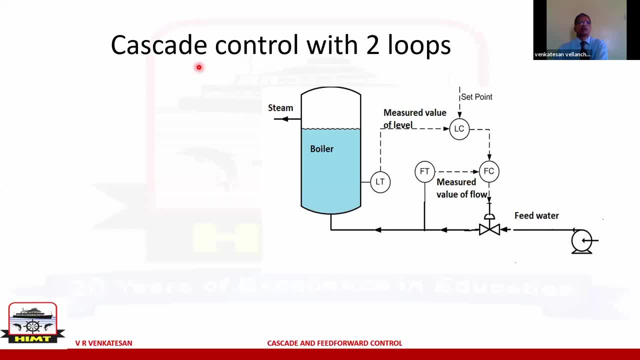 Like from one level to another level, then one more level, A series of falls That is called as a cascade. So cascade control is a serial control Where you will have two loops, sometimes more than two loops. There will be a master loop. 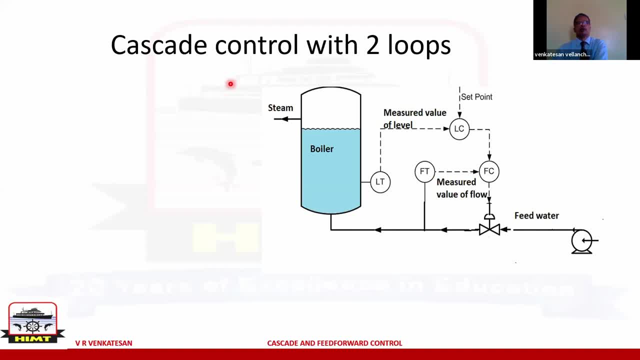 and there will be a slave loop, Or you can say main loop and a sub loop, And the control is executed this way. Once again, what is the variable that needs to be maintained? It is the water level. So is there a level transmitter? 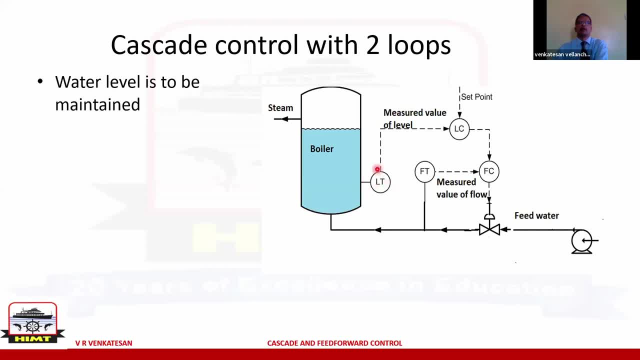 There is a level transmitter here. From the level transmitter the measured value of level goes to the controller. Set point is given. So the output of the level controller does not go directly to the feedback. Instead it is going to another controller. 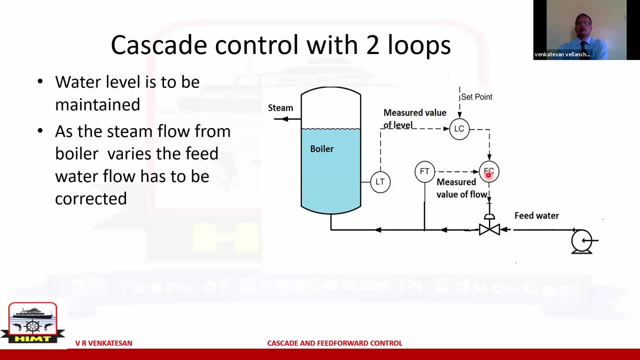 The letter FC means flow controller. So the output of the level controller goes to the flow controller And it is the set point for the. For the flow controller, the desired value of set points comes from the level controller. What is the job of the flow controller? 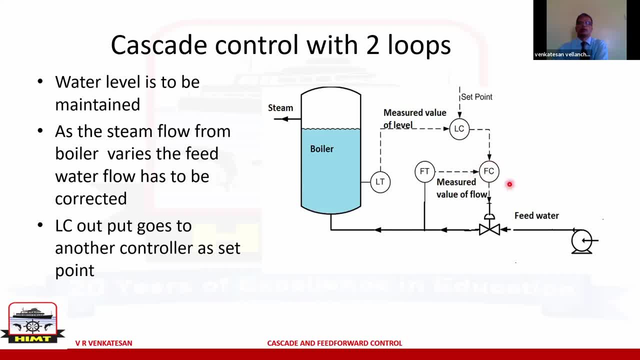 Is it a full-fledged controller? Yes, Its job is to maintain flow of the water- feed water- So will it need to measure the water flow? It is measuring like this, You see FT- FT stands for flow transmitter, So the water flow is measured. 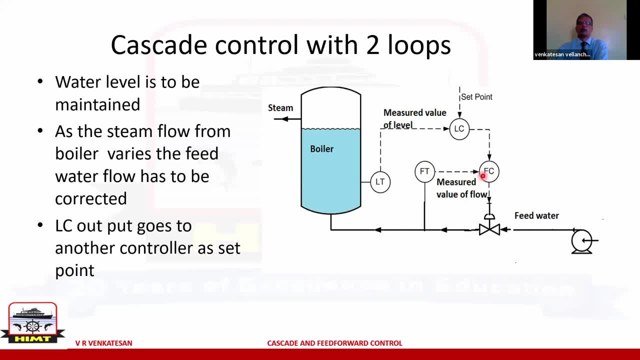 Measured value of water flow goes to this controller. Where is the desired value coming from? From the level controller LC? Yes, From the level controller's output it is coming. So the master's command is the Set point for the slave controller. 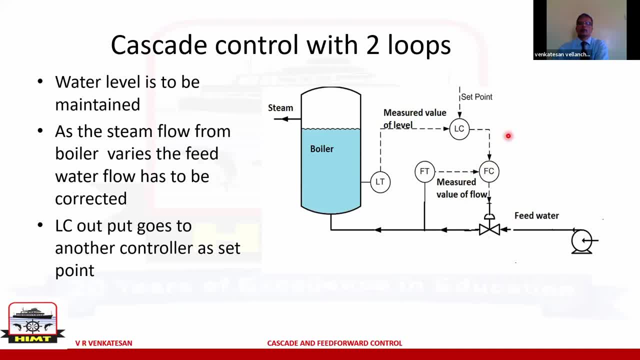 So this is a sub-loop control. What will the operator set? I want to change the boiler water level. Instead of 50%, I want to make it 60%. Where will I make the change? Set Set point. Set point of the level controller. 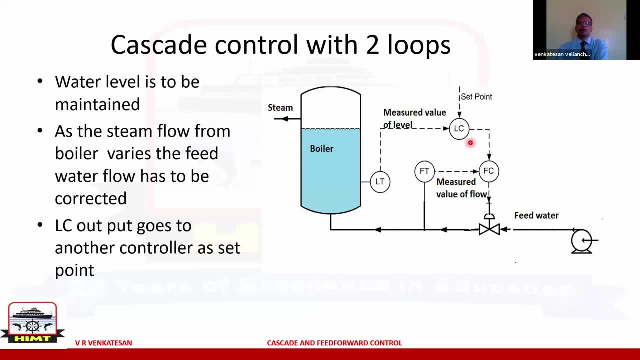 You have to make the change here. Yes, sir. Now the advantage of this system is you are using two controllers: One level controller, another flow controller. But what is the control variable? Are we trying to control the flow of feed water? 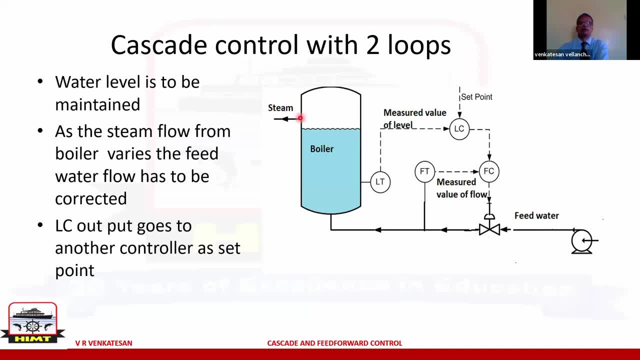 Or are we going to control the level of the boiler Level, of the boiler Level of the boiler? In this example also, the only variable we are interested in controlling is the water level. But to vary the water level you must change the 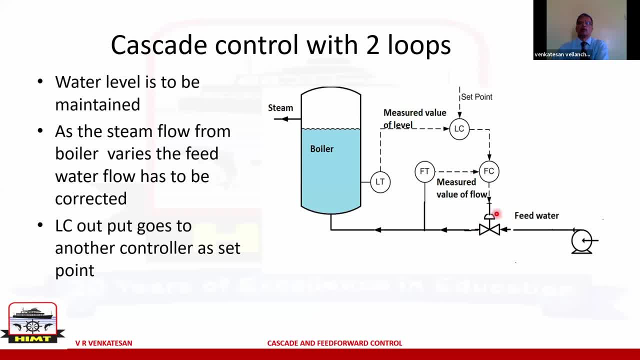 You must change the feed water flow And you have employed one more controller exclusively for controlling this. This is the example of cascade. So this is a Level control is the master loop And flow control is called as the slave loop or the sub-loop. 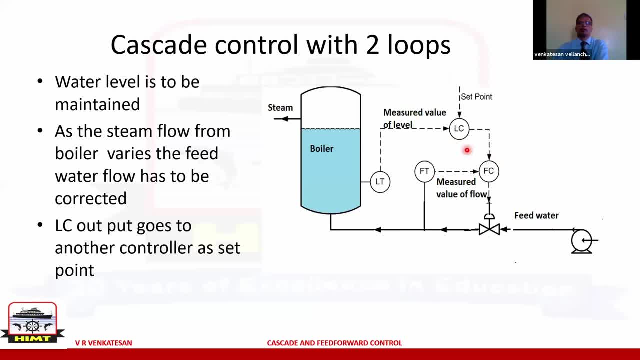 So there are two controllers you are using. It is definitely more expensive involved, But there are some benefits You can see. So, for example, if this valve is not opening freely, what will happen now? The way this is going to open is. 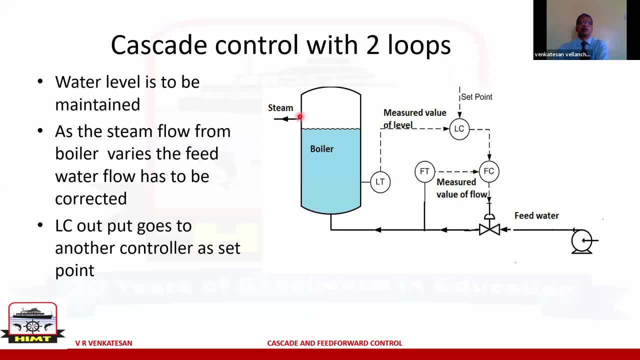 if the steam flow increases. steam flow increases, water level will drop And the level controller will increase the output. It wants to increase the opening of the feed valve, But the feed valve is not moving freely. What will happen then? Output of flow control changes. 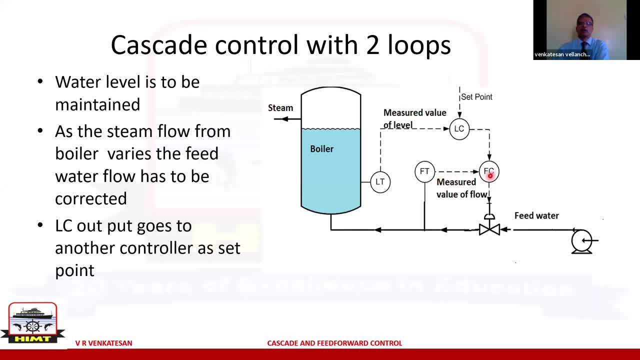 This: The desired value of flow is increasing, But the measured value is not increasing because the valve is ticking. So this, The flow controller itself, will increase its output. It will take care of its problem In the previous example. this problem will result in: 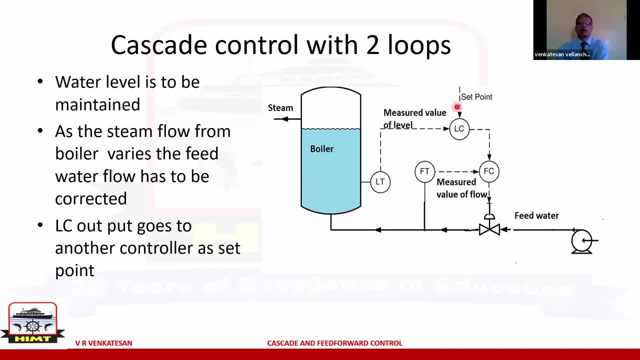 water level dropping And the master controller or the level controller has to take care of Here. a problem like valve ticking, which is called as a sub-loop issue, will be solved by this controller itself. Similarly, if there is a linearity problem, 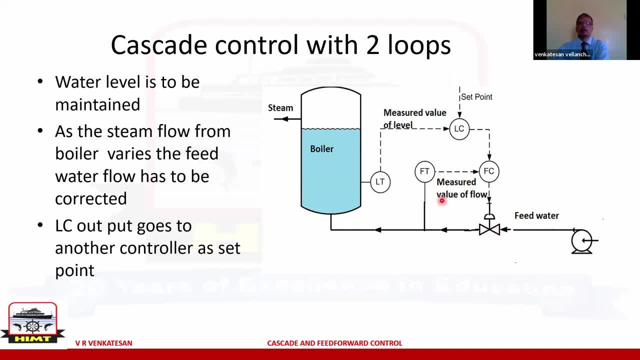 I open 10 percent, but the flow is increasing 20 percent. So what will happen then? Can this controller correct it? Water level will increase. No, no, But see, the point is the flow is being monitored here. 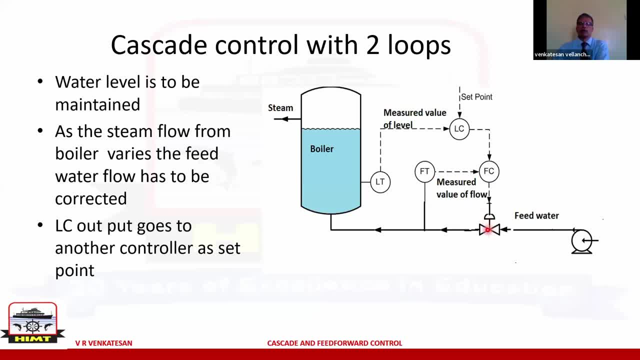 So if the So, it will close the valve. It will immediately close because it is monitoring the water level. Yes, Sorry, It is monitoring the water flow. Water flow, yes, Yes. So if the valve is not opening, 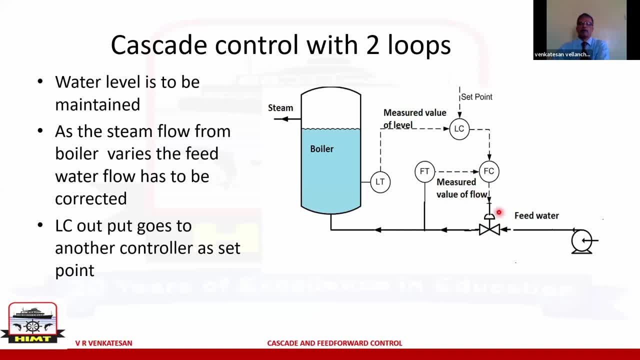 because of ticking, that will be solved. Same way, if the valve is opening little bit, flow is increasing too much, then also it will be solved. So any kind of non-linearity problem or imagine problems of Think, like for example: 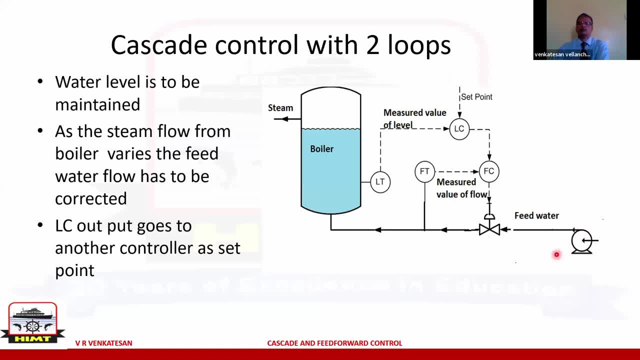 the feed pump is flowing down, Then feed water pump is flowing down, So will this loop take care of that? Yes, sir, It will take care of that. The valve will open more Exactly Because the flow is being monitored. 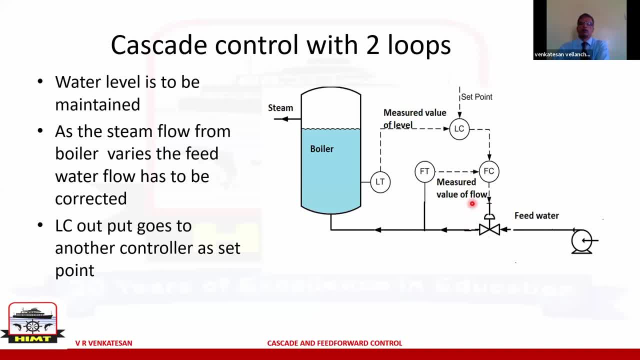 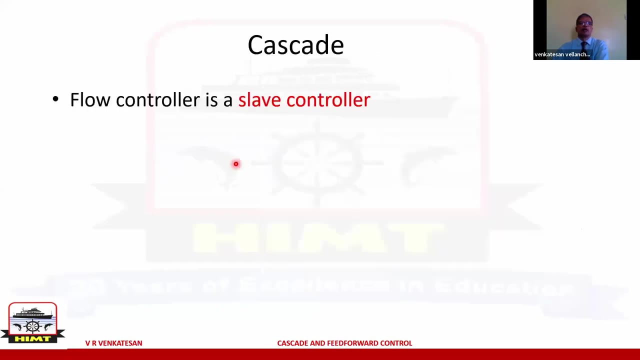 That is the advantage of this system. So disturbances which are affecting feed water flow will be solved by this loop. So you can see the advantage of having this. Level controller is called as the master controller And flow controller is called as the slave controller. 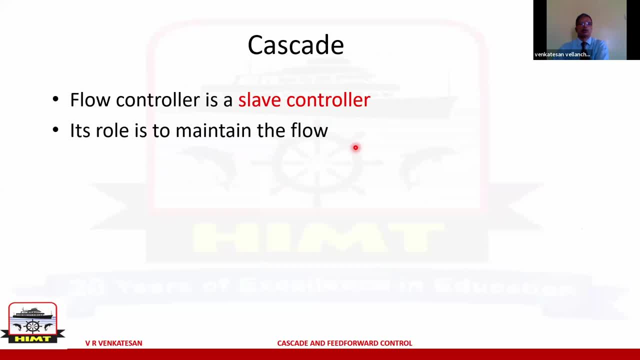 And if the slave controller's role is to maintain the flow under steady steam flow. if the feed water flow is disturbed for any reason, like the pump is flowing down, the correction will be immediate Because the water flow is being monitored. 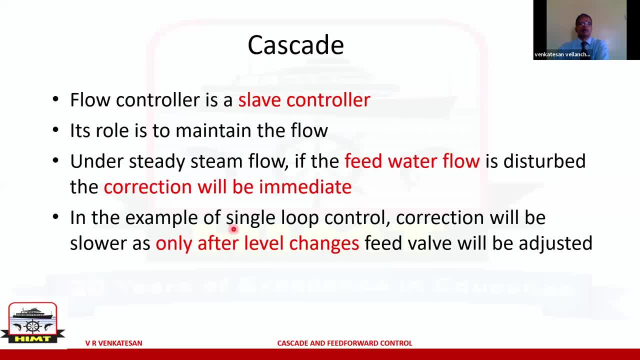 What will happen in the previous example: Correction will be Only after the level changes. That was the problem, Because you are monitoring only the water level, And if the feed pump slows down, then water level will drop and the correction will take only after that. 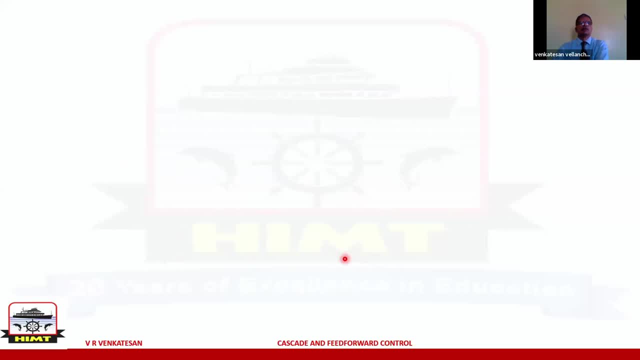 This is the advantage: You can call the feed water flow as an inner loop with its own controller. Water level controller is called as the master loop, So since the slave controls the inner loop, issues in this loop will not be affecting the level controller. 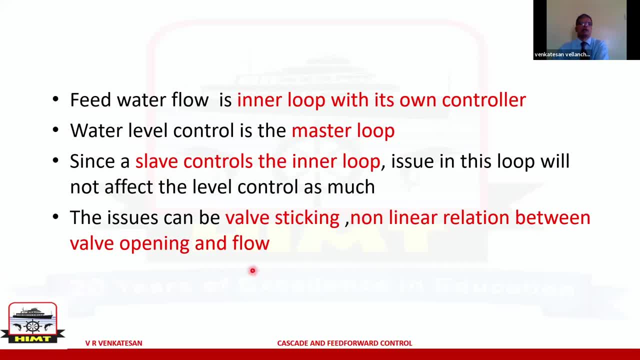 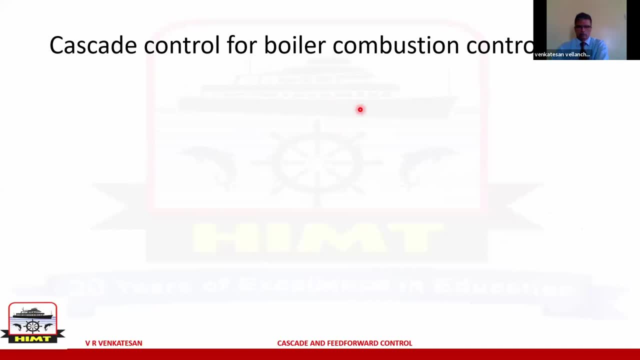 All these examples valve sticking, non-linear relation. So you have cascade control for boiler combustion control as well. What is the control variable for combustion control? Is you want to maintain the steam pressure? So in this case you can put steam pressure controller as the master controller. 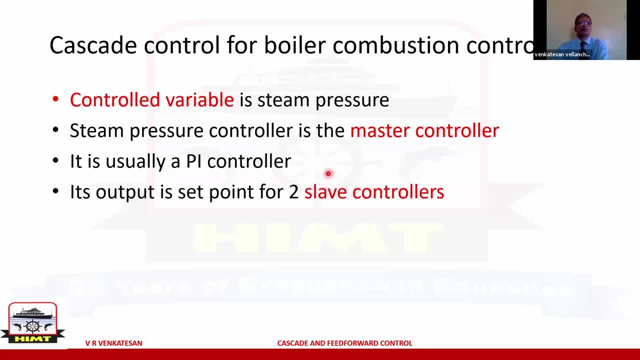 It is usually a P plus I controller. Output of this controller will go to two slave controllers. One slave is for fuel flow, Other is for air flow. So the idea is, if the steam demand is more, you must increase the firing rate. 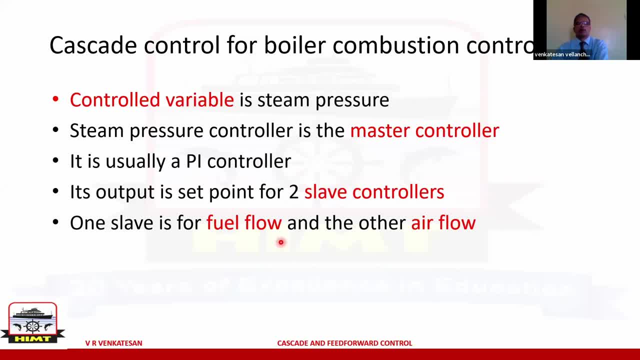 More fuel should be burnt. Along with more fuel, more air also has to be supplied. So both these loops are taken care of by two slave controllers. You must remember: fuel flow and air flow are called corrected variables. What is change? 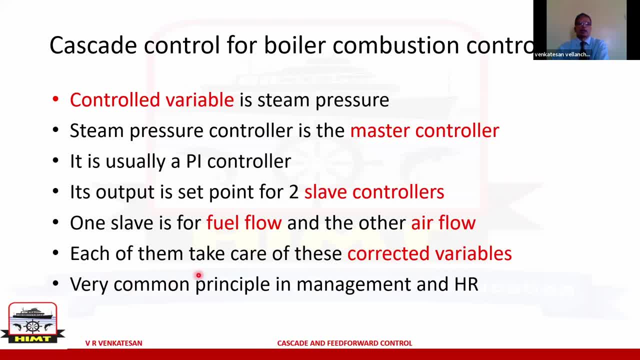 Now, this kind of cascade control. we will look at that picture. But this kind of cascade control is also very common in human activities. What is the meaning of delegating jobs? When you say job is delegated, what is the meaning of that? 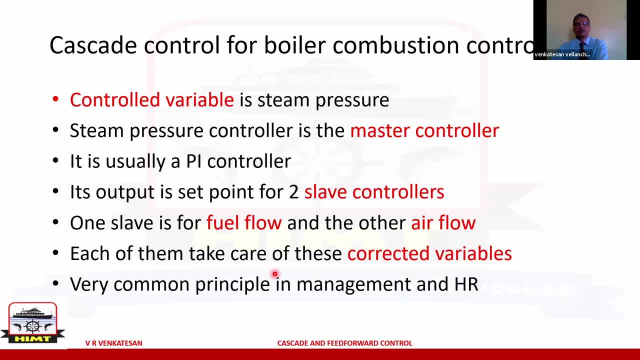 Signing up. The job is distributed Like onboard your vessel. chief engineer is there, Second engineer is there. Then watch keeping engineer is there? Ratings are there. Is there some kind of cascade control there also? Yes, sir, Everybody has their job. 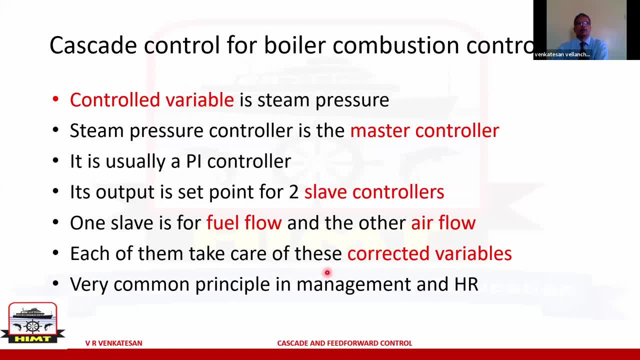 So there is a job to be done. For example, chief engineer's instruction is that today balance pump must be overhauled. That instruction will it be given to the fitter or will it be given to the second engineer? Second engineer. 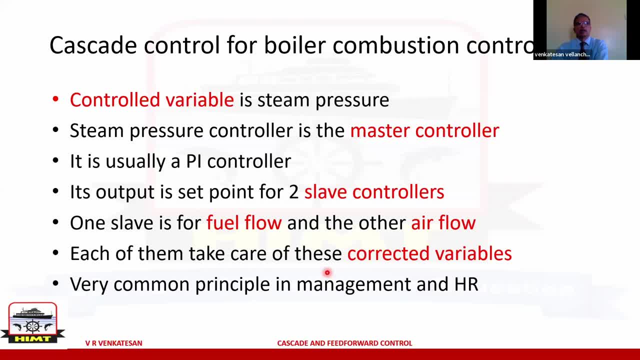 It is an instruction to the second engineer. Based on that instruction, the second engineer will have all the other crew and engineers at his disposal And he will be able to do what is required. For example, Right sir. For example, you start the job with: 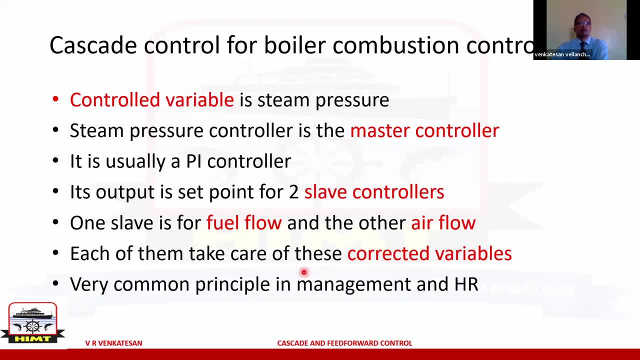 two persons, One engineer and one fitter, And the job is not progressing fast. What will the second engineer do? He will add one more person, Will he? Should he call the chief engineer and say: Sir job is not going smoothly? 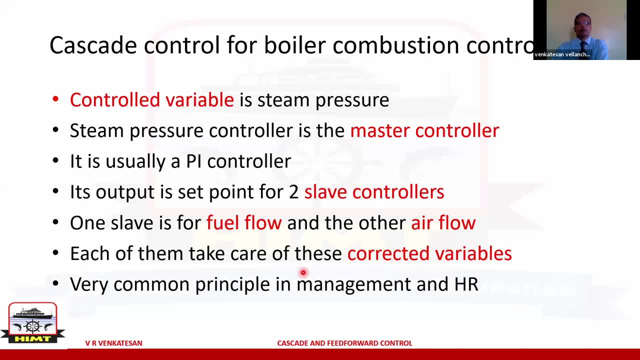 Or is he supposed to tackle it himself? He will delegate, sir. So if two people are not able to complete the job, second engineer will put more people on the job. Sir, Are you understanding? Are you understanding? So that balance pump overall is a sub-loop? 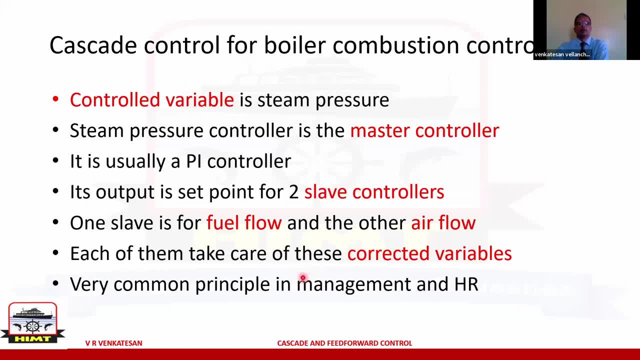 Second engineer is supposed to monitor the job and take corrective action as required. Chief engineer's only requirement is that the pump should be over by the end of the day. Right First, you open a pump and you discover that there is a shaft which is damaged. 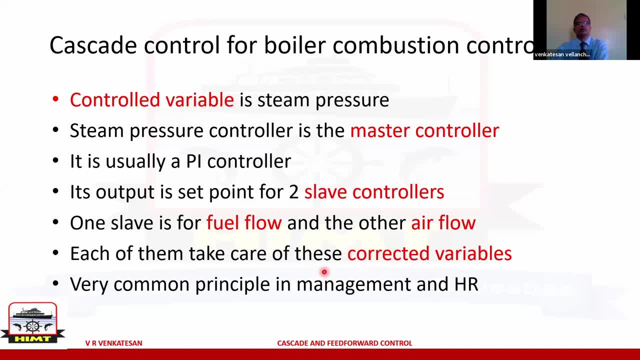 What happens now? Shaft requires replacement. Will the second engineer change the shaft himself or will he inform the chief engineer that shaft is damaged? He will inform the chief engineer Because in a general principle, changing a major part, you will have to consult the chief engineer. 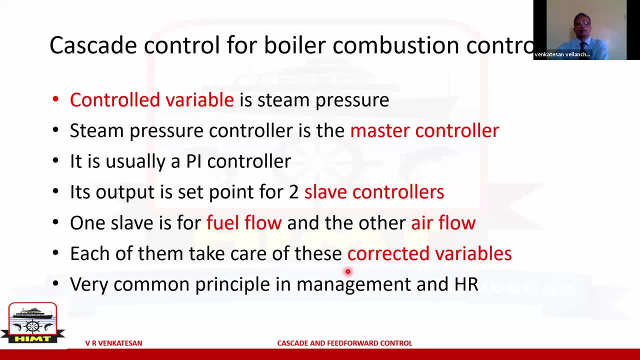 and take his instructions. So a damaged shaft is a. it is not a sub-loop problem. It has to be escalated to the master loop, That is, you have to take it to the chief engineer And then you take the decision. Are you understanding the principle? 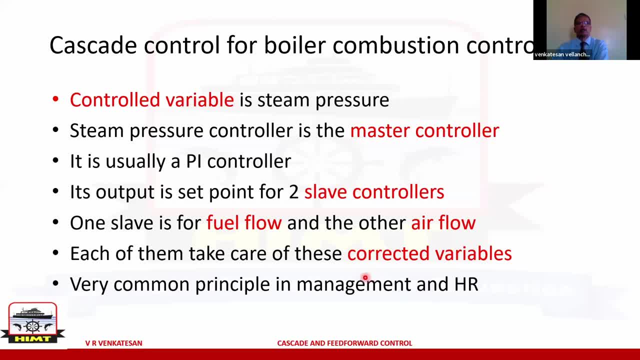 But putting more fitters, putting more engineers, that second will take care, Because that is called as a sub-loop problem. So these are very common principles used in a lot of applications. So if you keep that in mind, your understanding and engineering. 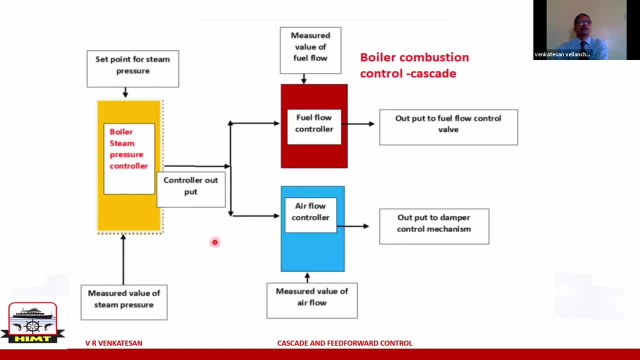 also will be better. So if you see this diagram shows like this: What is this part? This is the main controller. What is it telling? Boiler steam pressure controller. So you need a set point for this, Set point for steam pressure. 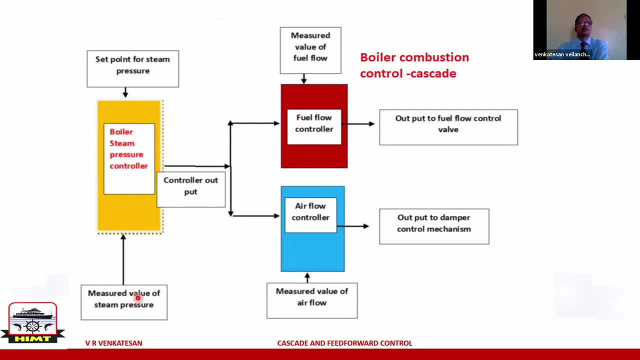 And you need measured value for steam pressure And the output will come. This is the controller's output. Where is this controller output going? Is it going to the fuel directly? No, it goes to air flow controller And air flow controller. 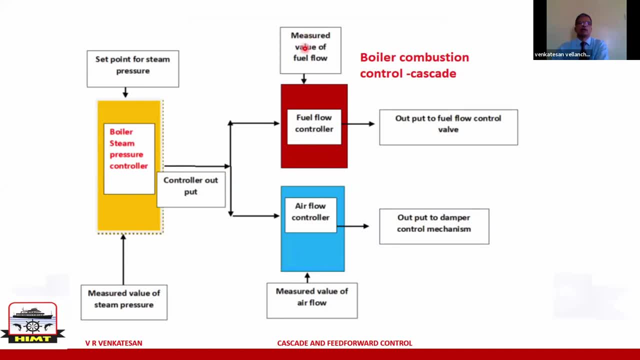 And actual fuel flow is measured here. Actually required fuel flow comes from here And the correction takes place here. Output to fuel flow control valve. How is the air flow controlled? Damper position: Damper position is there, So you have. 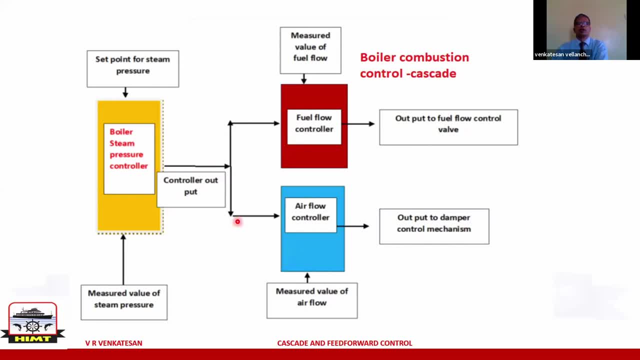 output of the steam pressure controller is coming to the air flow controller. Here the measured value of air flow comes. Desired value of air flow comes this way And then the output goes to the damper. This is also a very clear example of cascade control. 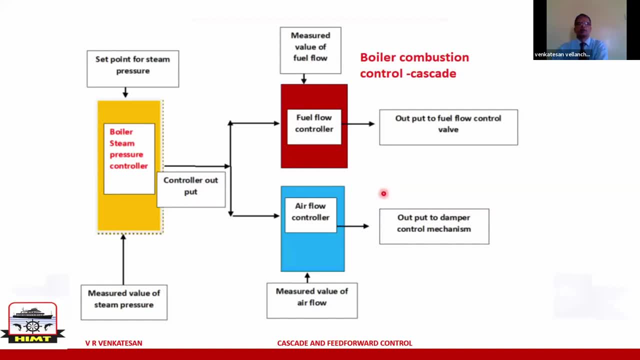 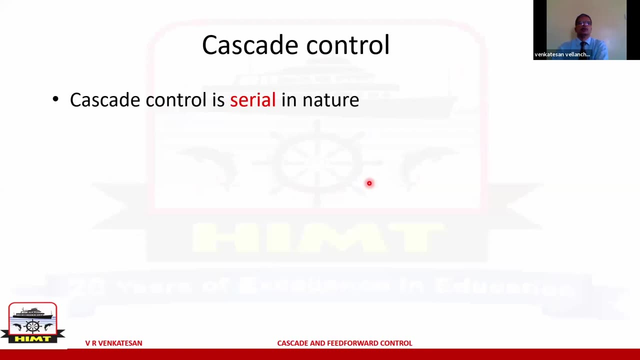 Widely used in boiler, Especially for tanker boilers or boilers which require, which are which drive machinery Like a turbo alternator or COPD. So these are a few points. Cascade control is serial in nature. The meaning of serial is the output of one control becomes. 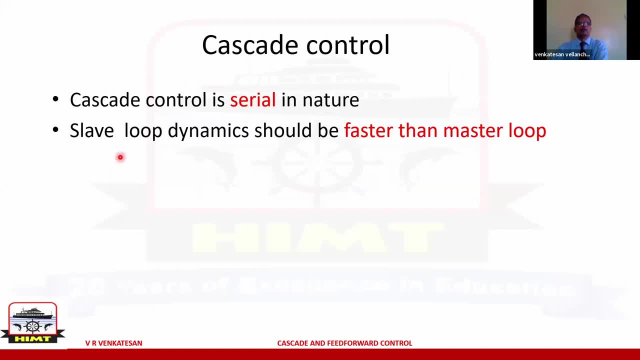 set point for the next controller. Slave loop dynamic should be faster than master loop. What is the meaning of that? This is what we said, That is, inner loop correction should take place fast. The controller itself should be faster than the master controller. 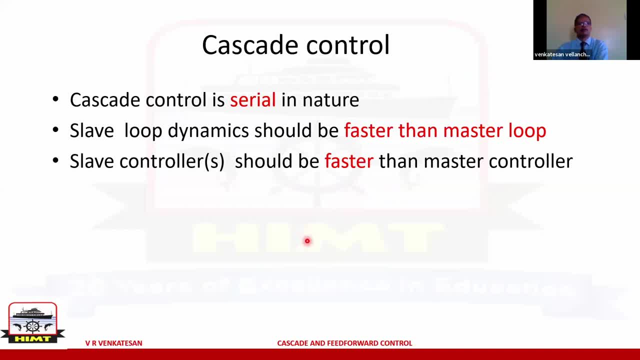 Does the same rule apply in HR functions also? What do you think If you are a second engineer? Yes, sir, it applies. If you are a second engineer, you have to take a step faster than informing the chief engineer If you can solve it by yourself. 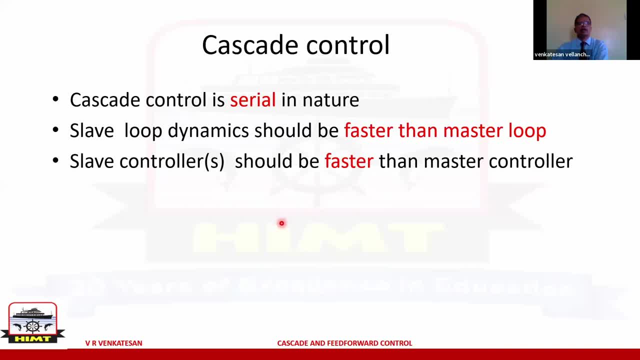 that's better. Yes, Ideal situation for most HR functions should be: your chief engineer should be a very relaxed person, And if you are a second engineer, your junior should be very fast, Right, sir? Then your life will be very comfortable, Right. 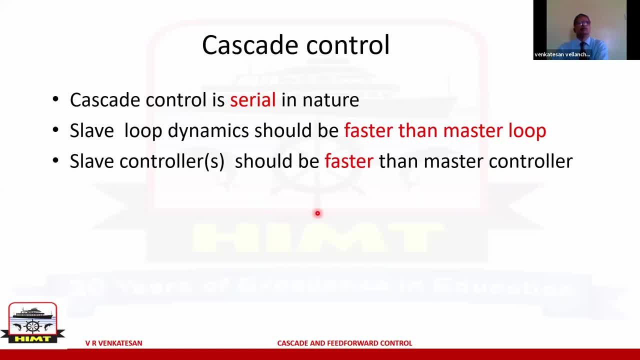 Unfortunately, often that is not the case. Often your chief engineer will be very fast and demanding And your juniors will take life very easy. Then the second engineer's life is not very easy. then For that there are other tuning methods. we will talk. 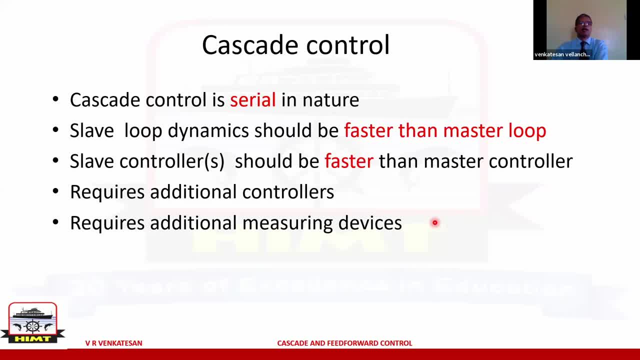 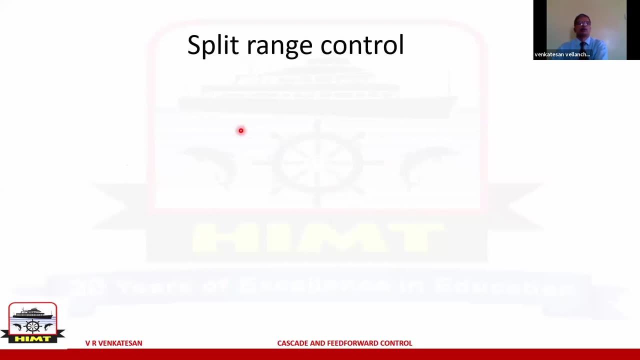 about in a different class. Alright, so there is this. additional controllers are required in cascade. It also requires additional measuring device. These are all the characteristics of this. You also have one more type of control. This is called a split range control. 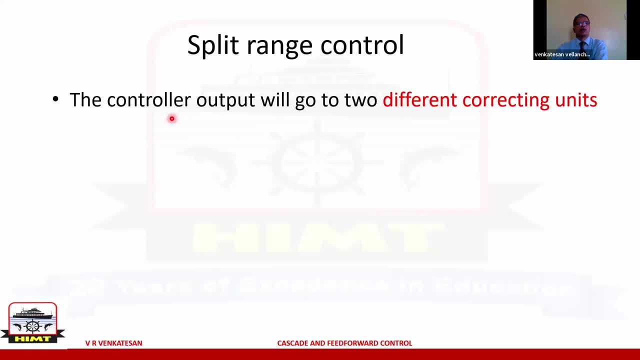 Here the idea is the controller output goes to two different correcting units. So the controller generates one output, but it will go to two different correcting units. The output will have two ranges. For example, if a controller output is up to 20 milli amperes. 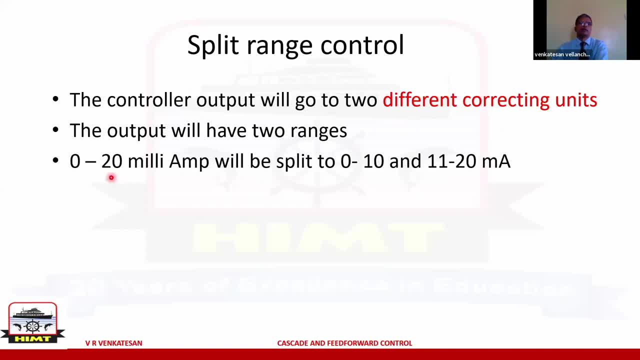 it will be split in two, Two ranges. It can be from 0 to 10 or 4 to 10, like that. it will be there And the upper range is divided like this: Then one range operates one correcting unit and the other range. 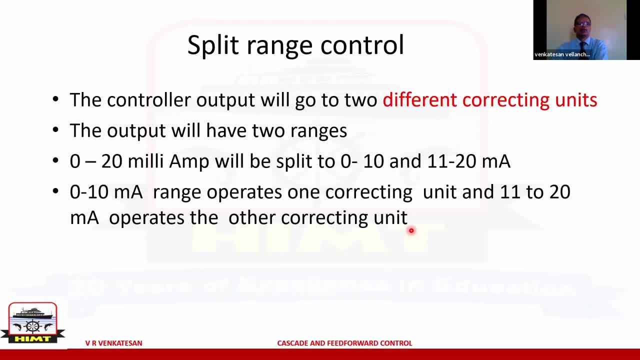 operates other correcting unit. If you see an example like driving, how do you control the speed of your vehicle? What are the two correcting units? Brake and accelerator. One is the accelerator and other is the brake. So when do you apply the brake? 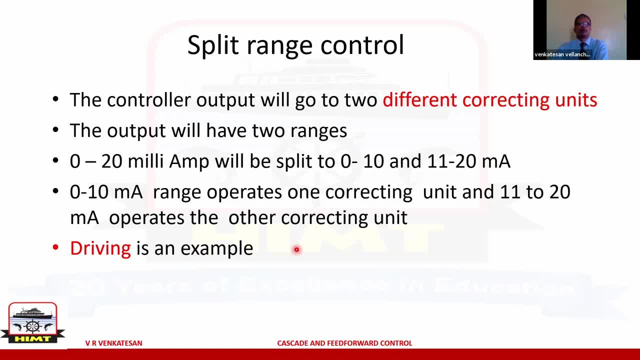 What do you do to the accelerator? before you apply the brake Reduce, You reduce the accelerator to minimum. Only then you will start applying the brake. Before applying the accelerator, brake must be released. So that is an example of this. You can also have example like air conditioning, where shipboard air conditioning is, is it? 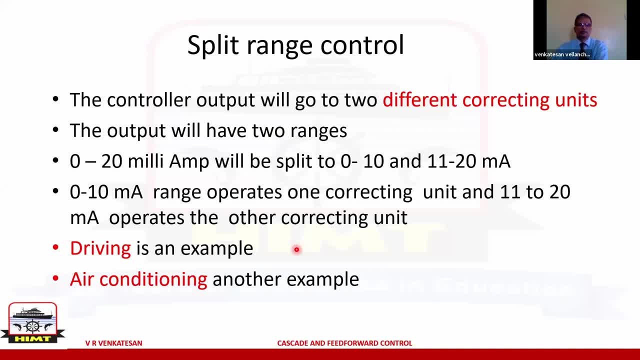 only cooling, or is it also involves heating, Involves heating. So before you start heating will you stop cooling? Yes, sir, Yes, only after you stop cooling fully, the heating will start. So these are all simple examples of control called split range control. 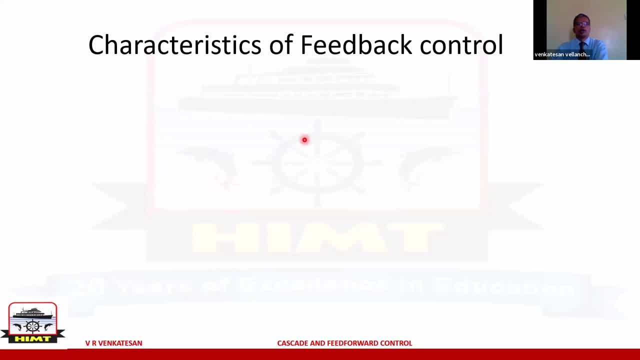 So what we have seen so far up to here, this is called error based control. where error develops and with an error developing, correction is taking place. So they are all called as feedback control. So example is boiler combustion, steam flow is the load. when steam flow increases pressure. 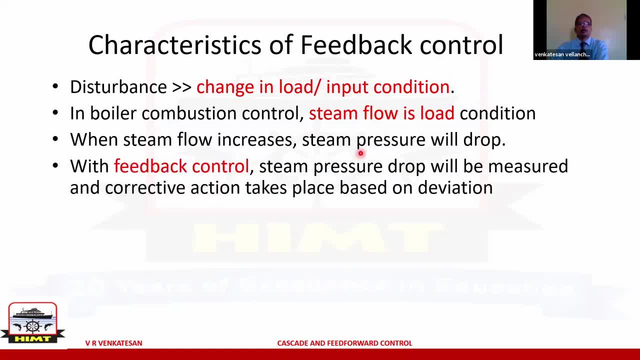 will drop. then, when the pressure drops, the drop is measured and corrective action takes place based on the amount of deviation. what is the correction? increasing in the firing rate. So this type of control is called as feedback control. Okay, So all the control you have discussed so far till now is called as feedback control. 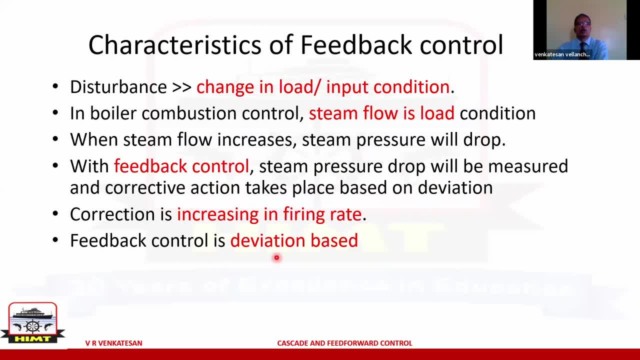 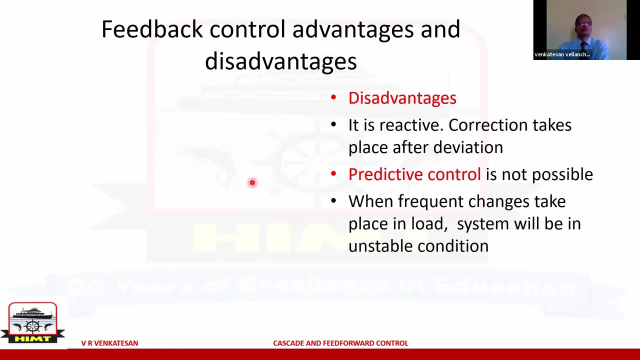 or also called as error based control or deviation based control It is. it is very widely used. it has got some advantage and disadvantage. Advantage is: deviation will result in correction, irrespective of the reason. what is the meaning of this? It does not matter what is the reason for the drop in water level or steam pressure. 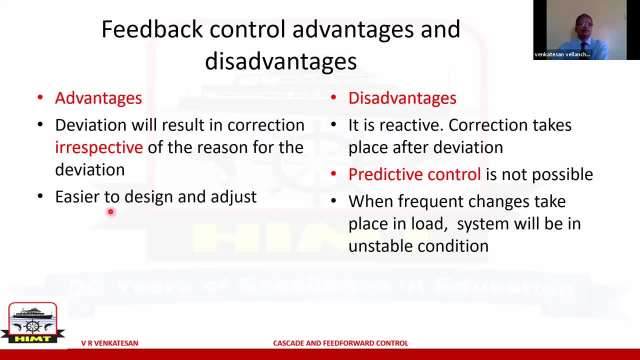 whatever may be the reason, correction will take place. It is also easier to design and adjust this part. you will see last class we discussed about how to tune PID controllers. Okay, And you can adjust this easily. Disadvantage is it is a reactive control, only after the correction takes place. sorry, 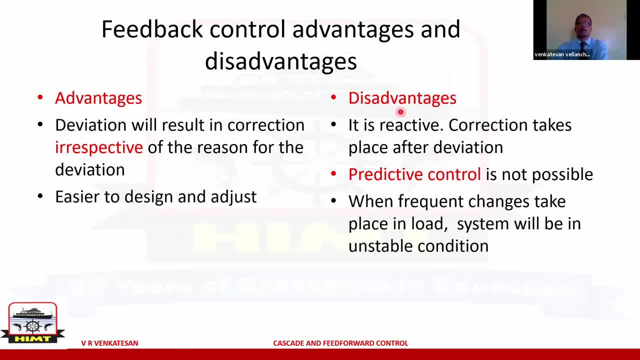 only after deviation takes place correction will take place. Predictive control is not possible. predictive means anticipating problems that will happen. So whenever frequent changes take place, the system can become unstable. Okay, So what is the answer to this question? 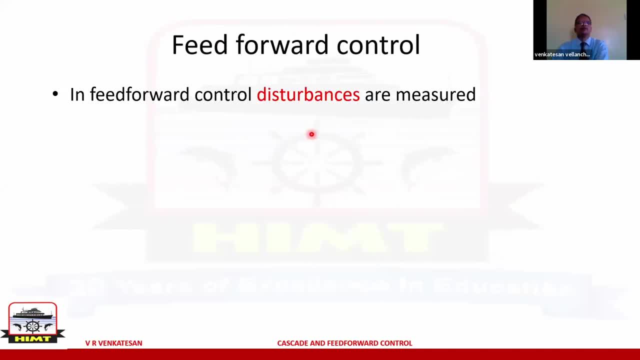 Excuse me, sir, Yeah, go ahead. You told that this is not predictive control. Yeah, But derivative is a part of anticipatory control, right, No, no, no, derivative is not anticipatory, because derivative is also. it is dE by dT. 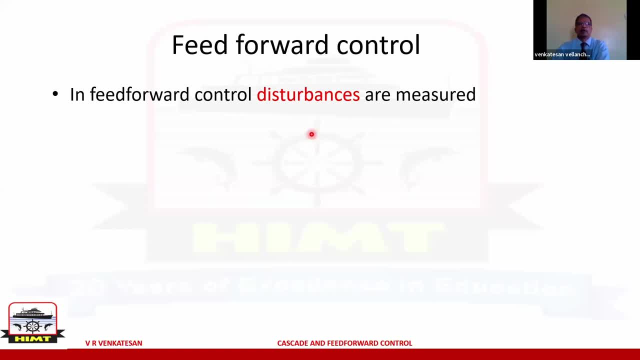 For the three. it reacts first. It reacts first, But it cannot do beforehand Error. even for derivative control, error has to take place, but it does not go by the value of the error, but it goes by the rate of change in error. 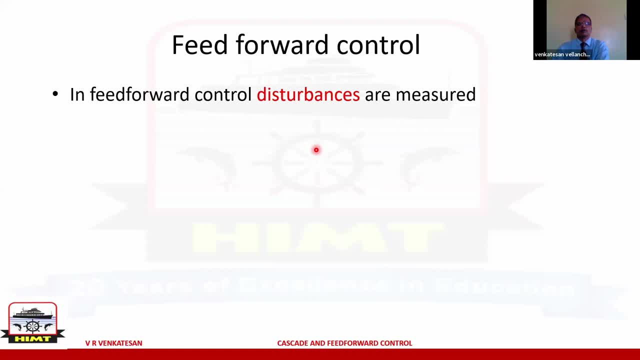 Do you agree? Thank you, sir. Okay, sir, So derivative control is also error-based. It is not. Good morning sir. Yes, please, Sir. we are heading towards the end of the session. Thank you, sir. 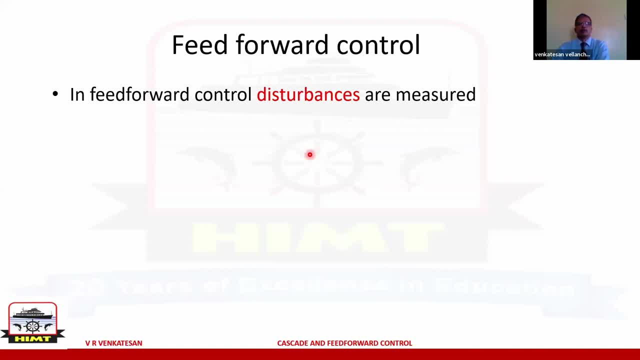 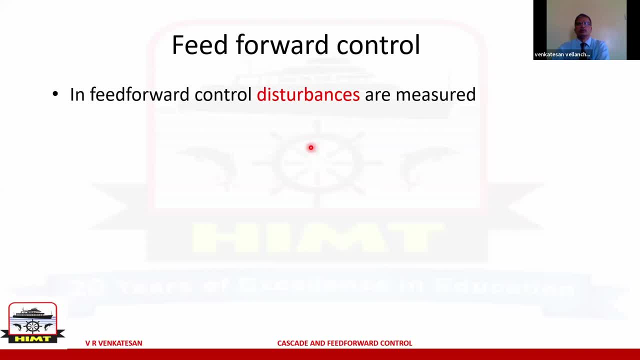 20 milliamps. Now, why not from 0 to 4?? It's why we leave the 0 to 4 part. That is because for for to create any movement, you need some reserve in your pocket. Yes, sir. 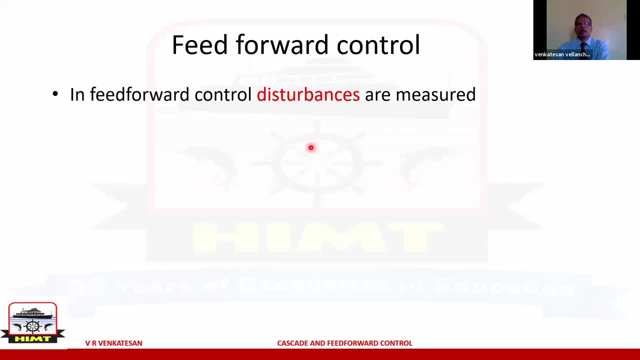 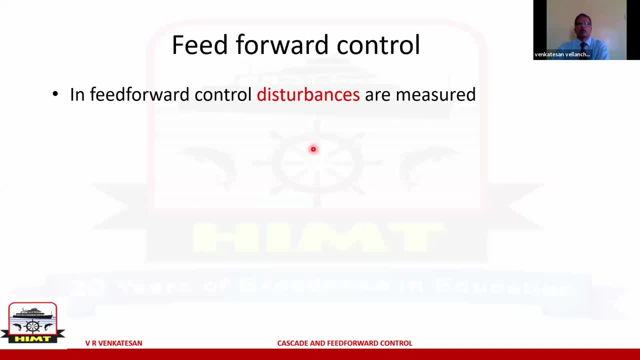 Thank you, sir. So the value of the valve is 0, right, Yes, sir. For example, if I mean to say that only by zero current the valve will reach its close position, you cannot make the current less than zero. no. 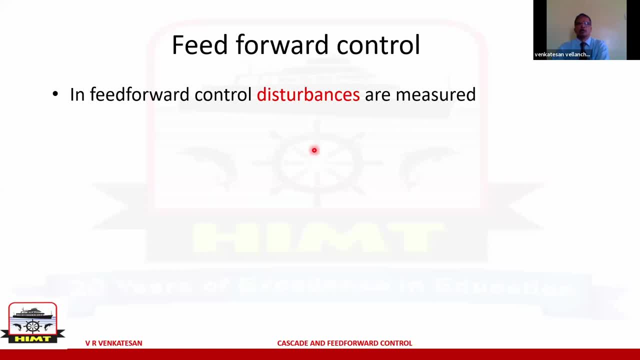 Yes, sir. So you need you both ways. you need a, you need a cushion In the sense that, before my output reaches its maximum possible value, the valve should be at its either end, Whether it is whether it is fully open or fully shut. 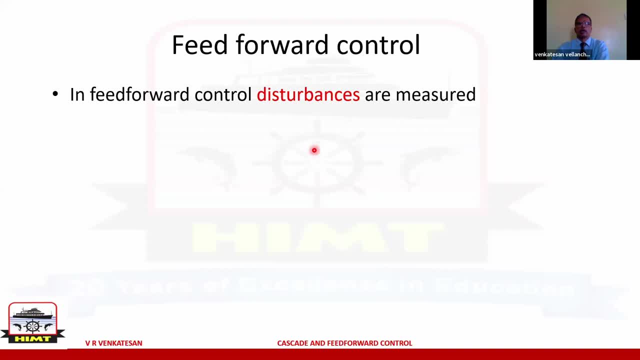 shut. you should be reaching it before the maximum possible value of the controller is reached. So controller can actually vary the current from 0 to 20, not 20, sorry- 0 to 24 milliampere 0 to. 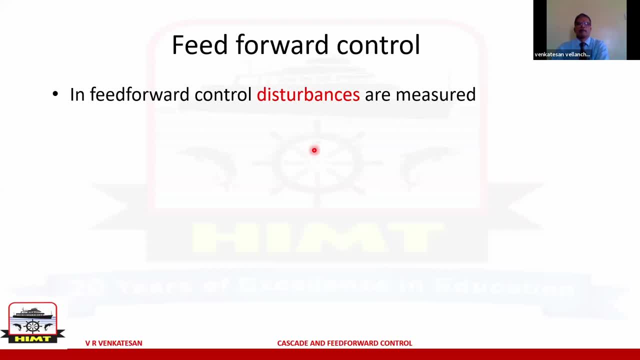 26 milliampere, the current will wake up, But the actuation should be set to 4 to 20 like. Okay, sir, Thank you, That is always the case. Any output should not be at its extreme level, should reach the actuator at its extreme level. 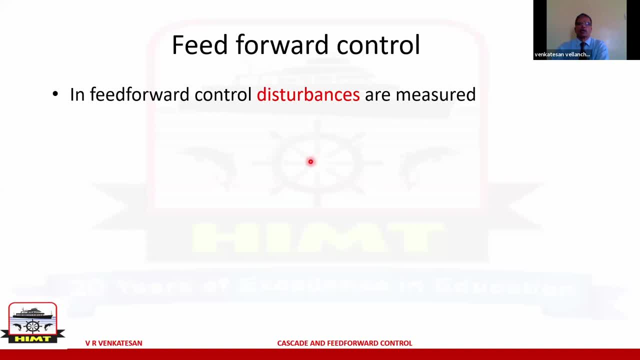 Thank you, sir. The extreme levels of the actuator should fall in the extreme levels of the controller output. Yes, sir, Excuse me. Yes, We are Venkateshan sir. Yes, Here one question from Jagat: In boiler is split range control used? 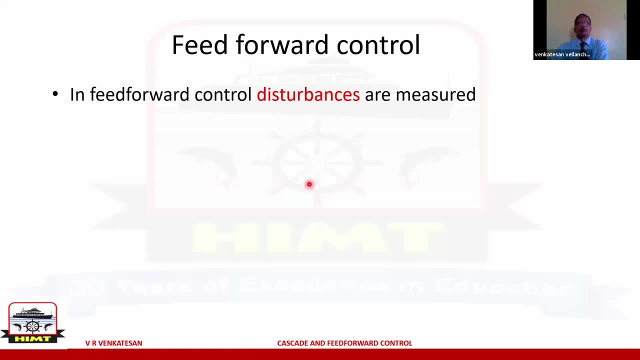 No, Thank you. Split range control is normally used when you have two different actions to take place, Like sometimes. you can use it for jacket cooling water If the jacket cooling water requires normally. jacket cooling water requires cooling or heating- Both. 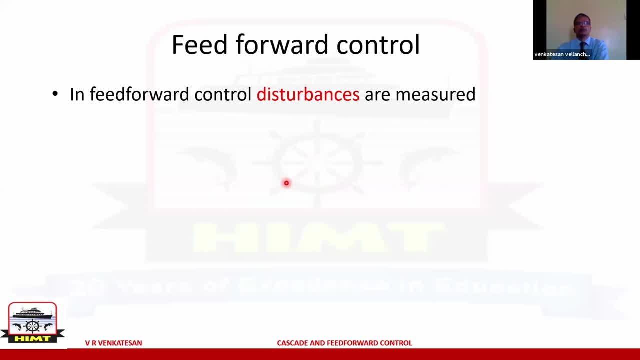 Cooling, sir. Cooling- Your normal understanding of jacket cooling water is for cooling right Both, Both heating and cooling. But the heating function normally is not controlled. It is manual Normally in many vessels. once a vessel is in port and the jacket cooling water heater is put into use, it is not an automatic or control function. 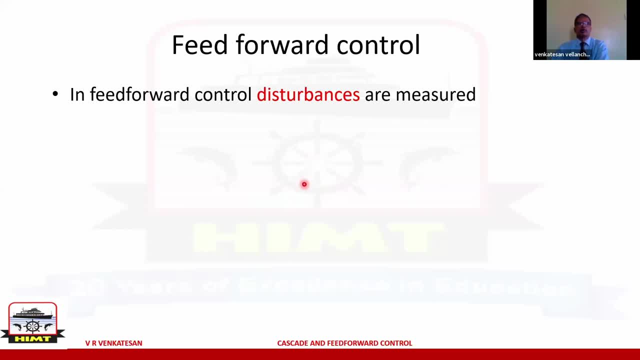 Yes, sir, Yes, sir, Yes sir. If you have a vessel, imagine, because if your port stays for long, can you allow the jacket water temperature to drop to some 60 degrees and then again start increasing when the vessel is sailing. This is something you can do. 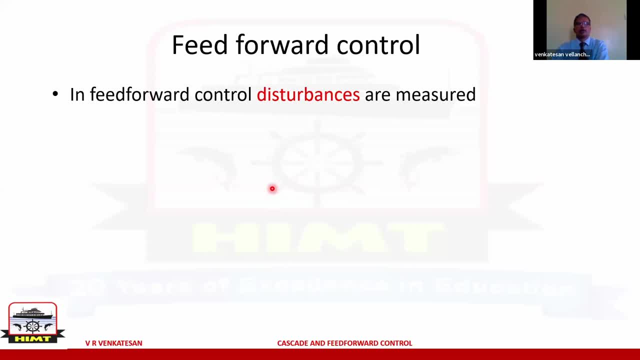 But suppose the vessel is in port for very short periods, Yes sir, Then it will be better to maintain the jacket water at a uniform temperature, even in port. In that case, what will happen is the steam heating will also be automatic. 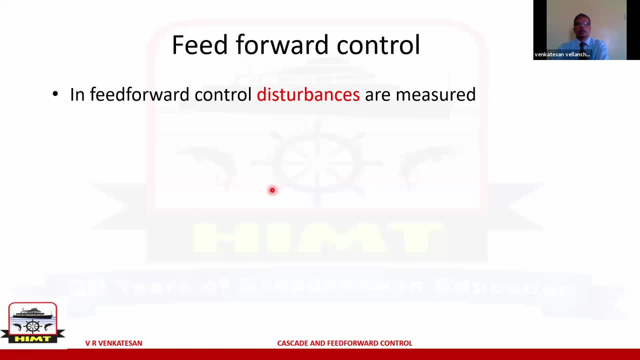 The vessel comes into port, cooling will be shut down and heating will start. You start the engine, heating will reduce and cooling will start. So you can do like that in the case of jacket cooling water system. Generally split range is used when two opposite corrective actions are required. 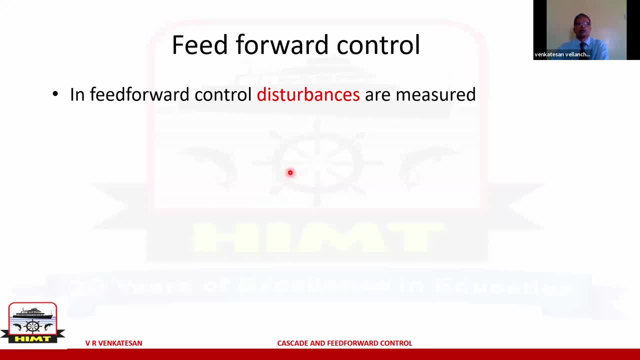 That is why driving is an example, or air conditioning is a good example. Okay, can we move on to this feed forward now? Yes sir, Yes sir. So in feed forward control, what is measured is the disturbance, What is the meaning of disturbance? 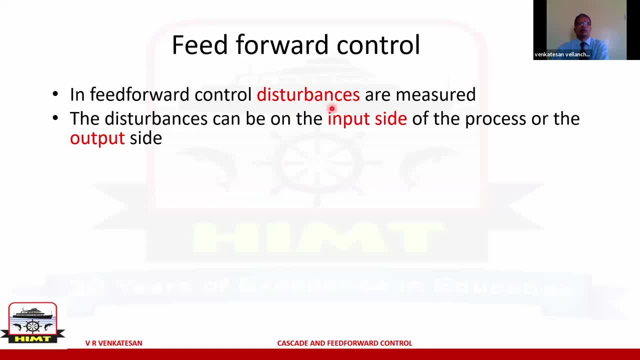 Disturbance means a change in a value. The disturbance can be on the input side of the process or you can have it on the output side of the process also. You will see examples. So in the same boiler, if the steam flow is measured, 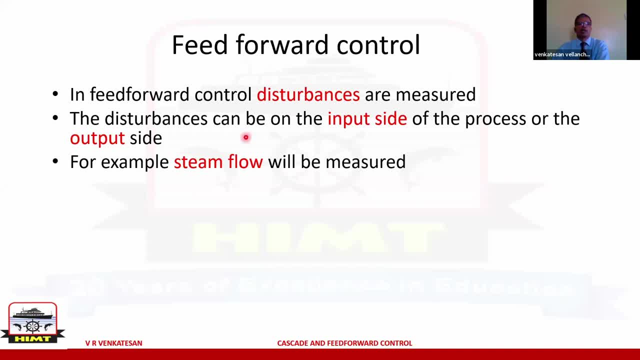 steam flow is on the output side. Yes, sir. So if steam flow is measured, and as soon as the steam flow starts increasing, if I increase the firing rate, can you do like this? Yes, sir, Yes sir, We have to increase the firing rate. 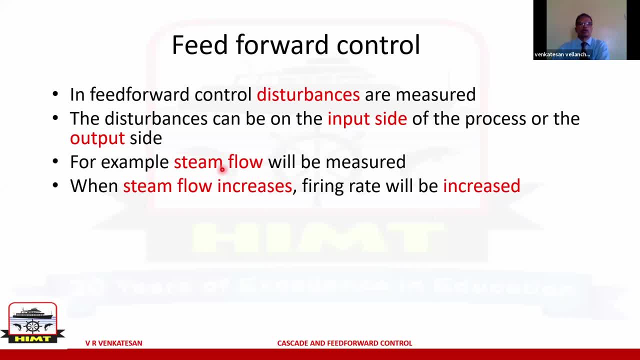 Yes, sir, We have to increase the firing rate. Yes, So can you not have a control where increasing steam flow will also mean firing rate is increased? It is possible to do like this. If you do this way, the correction will be faster. 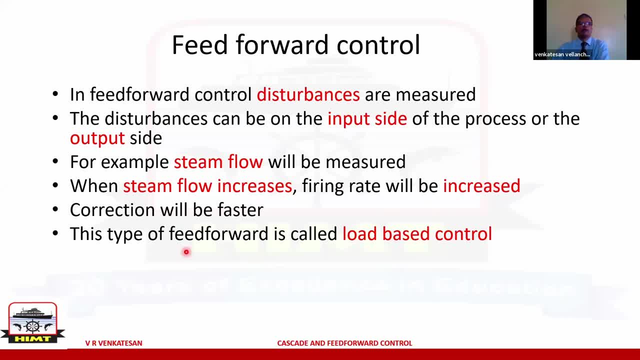 This type of control is called feed forward control. So when we said feed forward control measure, the disturbance steam flow is a disturbance in the output side. It will be like this: Excuse me, we are Venkateshan moderator here. 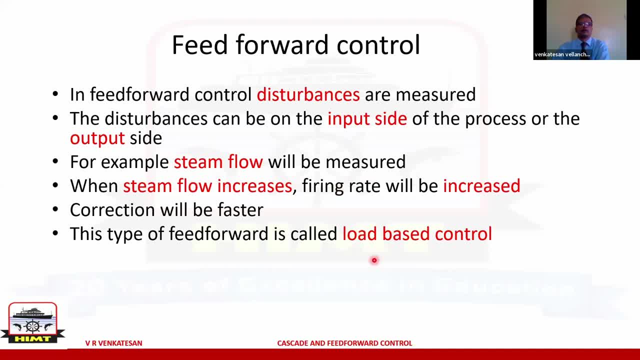 We have 10 minutes left for this session. We have 10 minutes left for this session, Thank you. Thank you, Sir. I had a doubt on this, sir. Sir, I had a doubt on this, sir. Yes, please go ahead. 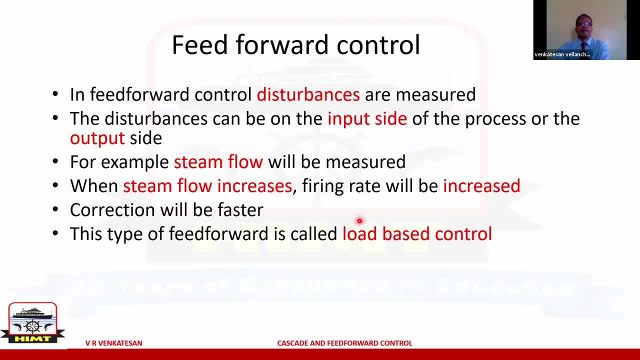 Yes, please go ahead, Sir, Go ahead. Does the water controller come into this part? Does the water controller come into this part, Like based upon the steam flow rate? does the water controller work? Is there any setup like that? 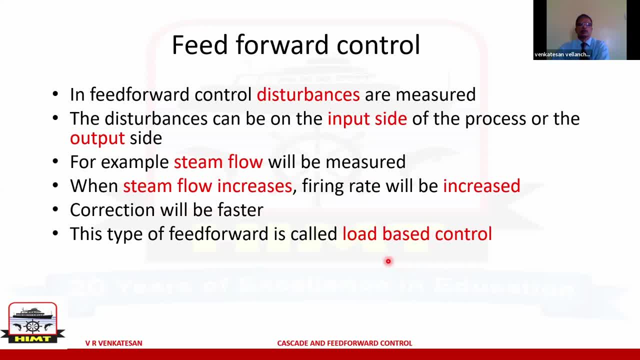 Definitely, definitely. It's very much there, Okay, sir. It's like steam flow is measured and firing rate is increased. Okay, Level is also measured. In fact, it is very common for water level, Because boiler water level has got this problem of 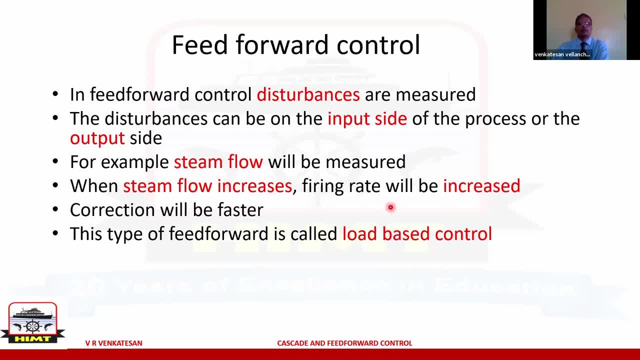 swelling and shrinkage. Okay sir, Okay sir, This feed flow controller solves what doubt I had, Like: does it really calculate your steam flow rate for the water controller to work? So now, this statement, I think, gives me the answer now. 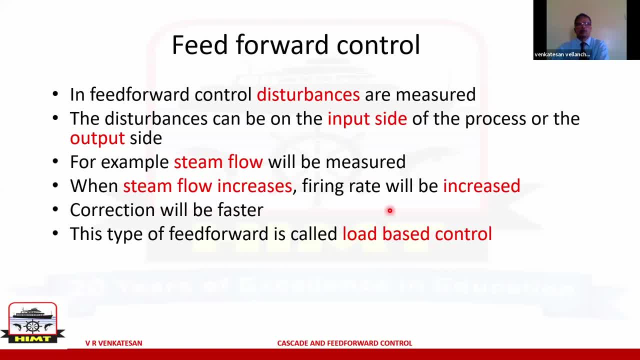 Yeah, definitely, Definitely. If you work in a tanker with a 16 gauge boiler, you will see that on the steam outflow line there is a steam flow measurement is there? Usually it will be a venturi venturi tube or an orifice plate. 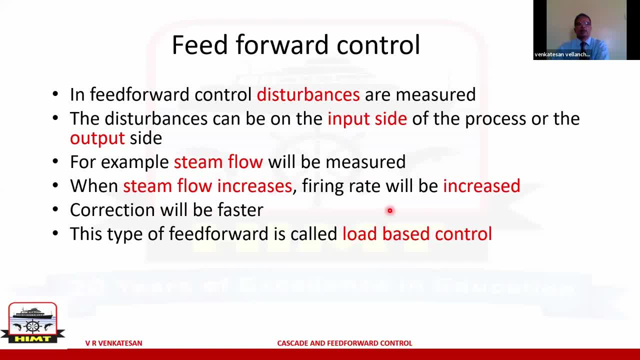 like that will be there. Exactly, sir. Arrangement is that as the steam flow increases, feed water will open more. Okay sir, Okay sir. So this type of feed forward is called load-based control. Why this is called load-based? 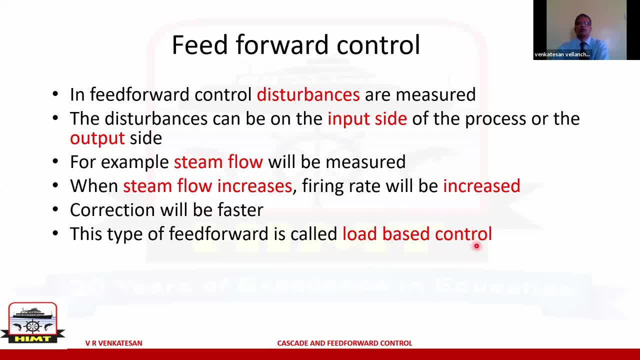 is because steam flow is the load And based on that we are controlling this. But feed forward control is difficult to use alone, Alone, in the sense that without feedback, if you want to control, it is not easy. The reason for that is: 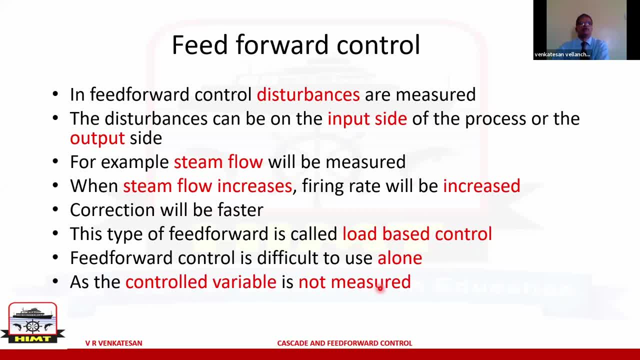 the actual control variable is not measured. What is the control variable for boiler? Steam rate, Feed water: No, no Controlled variable for boiler combustion, Fuel, fuel Fuel and steam pressure. Steam pressure: Steam Steam pressure is a control variable. 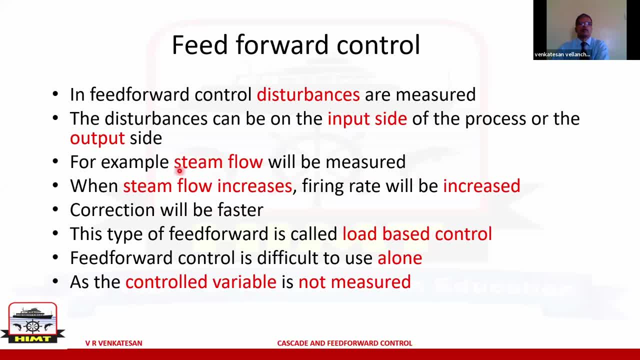 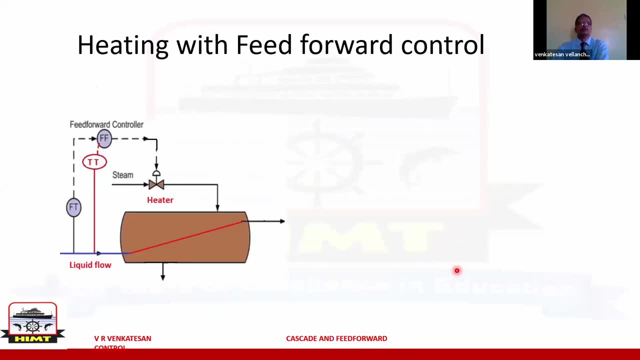 And here, what are you measuring? is the steam flow? Without measuring the steam pressure, it is not possible to control exactly. You will see example as you see. You take this case. This is an example of heating with feed forward control. What is the purpose of the? 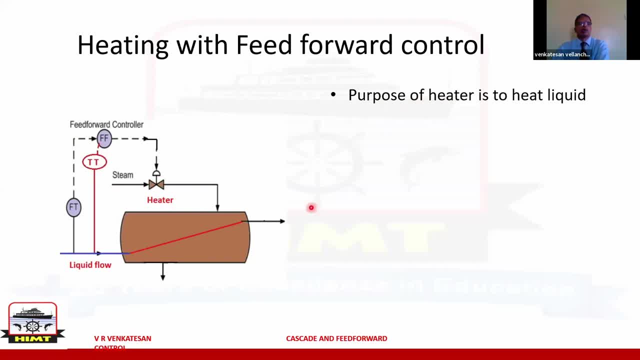 heater is to heat some liquid. It can be water or fuel or any liquid. Heating is done by steam. This is a steam heating valve. Suppose somebody says this is a heater and your job is to maintain the temperature of the fuel at, for example, it is a purifier heater. 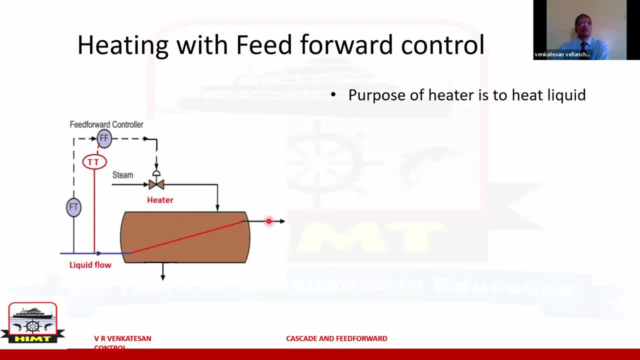 and you want to maintain the temperature of the fuel to 90 degrees- 95 degrees. Will you put a temperature sensor here? Yes, sir, can be at the output. That is what you normally expect. I should put a temperature sensor here and. 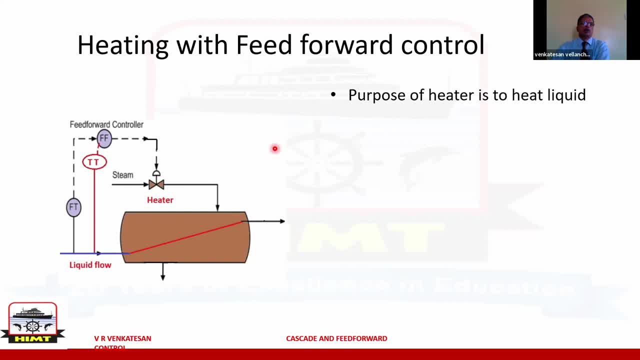 based on the temperature measurement, I will open the steam. If the temperature is less, I will open more steam. But see this case Here what is being measured is the oil flow. This is a flow transmitter. The flow rate is measured and sent. 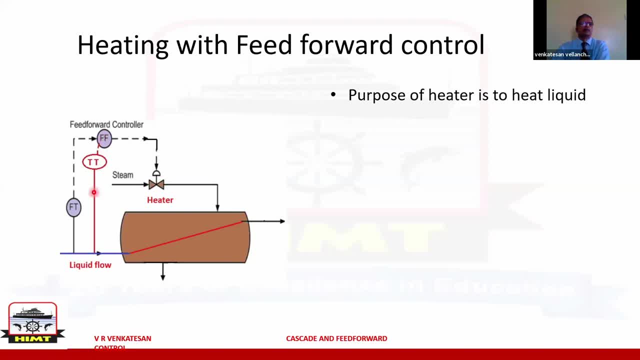 What is the red line? This is the temperature. So the temperature of the oil is measured. flow rate of the oil is measured. Based on these two values, will it be possible to decide how much to open the steam? Yes, possible. 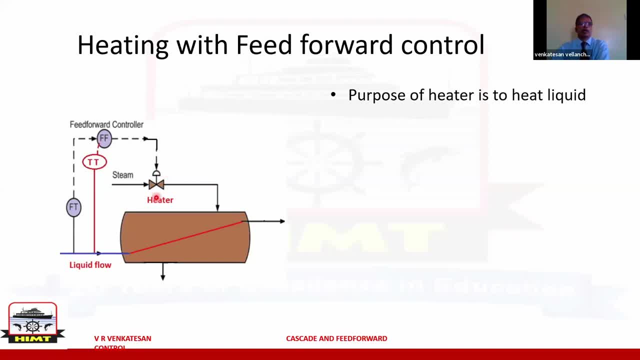 It is possible. So, based on that calculation, the steam valve will be open. Ok, sir, Sir, one doubt on that. sir, If your heater efficiency drops and the output temperature is not reached, even though you have set points- suppose 95, you have set at the purifier. 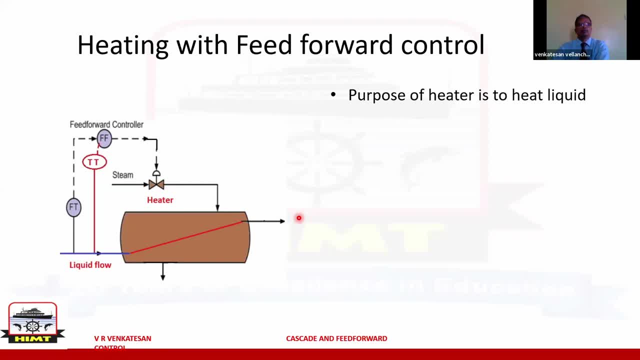 and the temperature has not reached. So then, how will you check on that error? That is the problem with this, because it will not take care of that. We said it is not easy to use it alone. Ok, sir, Your point is correct. If the heater efficiency drops, 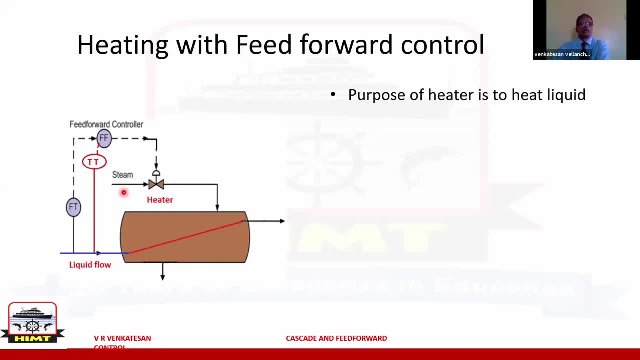 or even take a case the steam pressure itself drops. What happens then? Steam pressure drops, then also your efficiency comes down. Yeah, Steam pressure. Then your calculation has gone wrong. On what basis will you do the calculation is? you will expect that I am giving 6 bar. 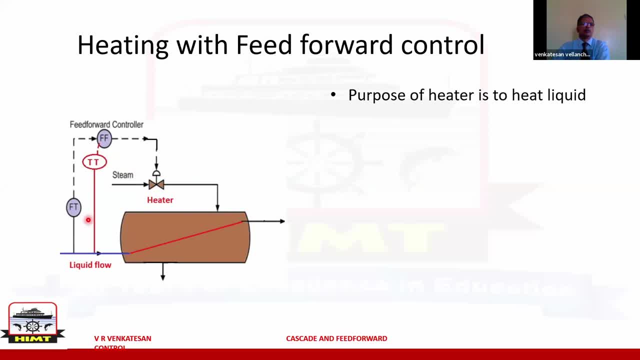 steam pressure here: 6 bar steam is here. The oil comes at this flow rate. Oil comes at this temperature. Based on that, the valve should be open 30 percent, If the see this is the meaning. Steam flow is measured. Ok, Control variable is: 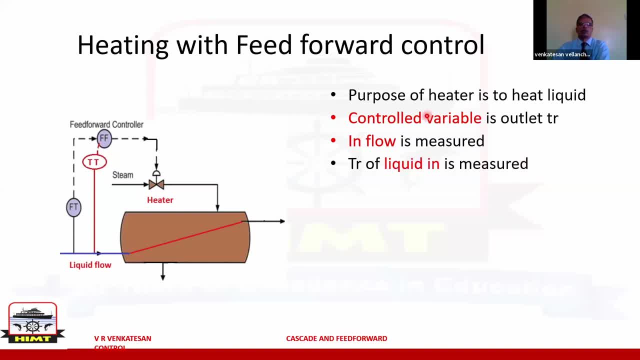 outlet temperature. That is what we want to control. Temperature of liquid is measured. So take this case: when the flow increases, what will happen? What will this controller do? It will open more steam. It will open more steam, sir, Like it will tell to more steam. 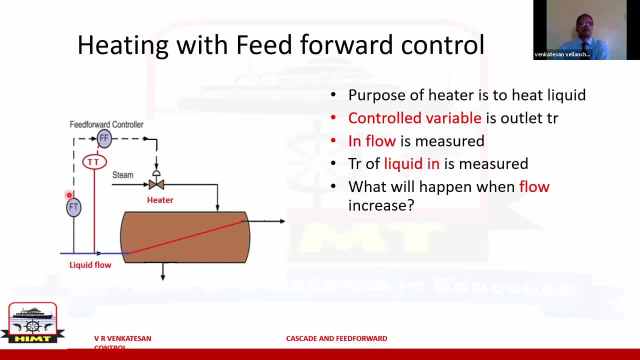 It will open more steam because the calculation is already there: For this much of oil temperature, I must open. like this, Same way, if the inlet temperature increases, what will it do? So it will solve this problem based on your accurate calculation. You have to calculate accurately. 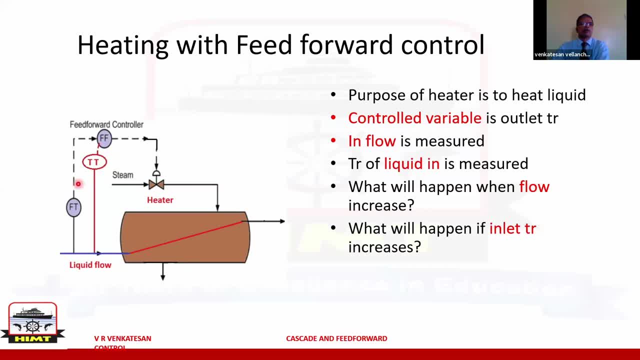 This is my heating capacity in the heater. This is the temperature at which oil is coming. This is the flow rate at which it is coming. You do that calculation and the controller generates that output. Now the issue is just like the point raised by the student. 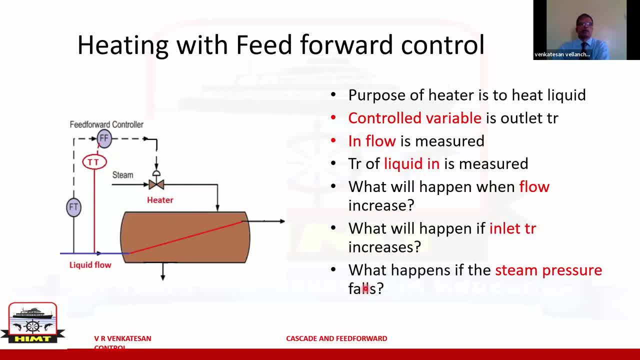 If the steam pressure falls or the heater is fold, then this controller cannot solve that issue Because you are not even measuring the output. You are not measuring the output. You are not measuring this. What is commonly done is that you need to put both. 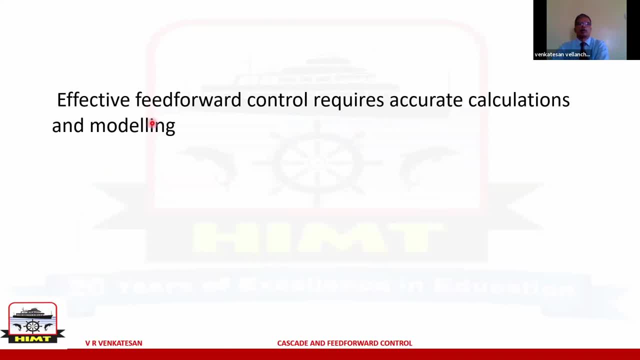 This is the reason we said effective feed forward control requires accurate calculation and modeling. The simple meaning is that you should know that for this much flow rate and temperature, this much heating is required If any unexpected change takes place- unexpected or what you have not taken in your calculation. 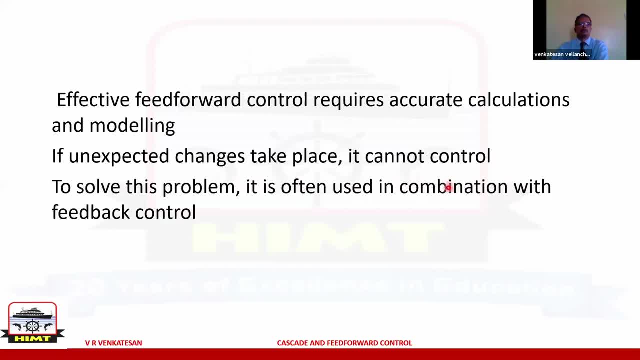 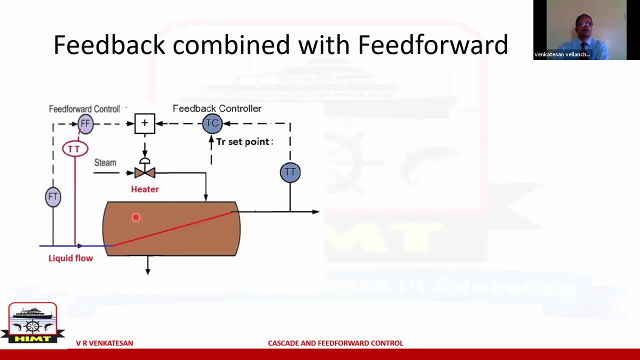 cannot do any control. That is why, to solve this problem, we use it in combination with feedback. So if you introduce feedback, it becomes like this: This part remains the same. This is the feed forward part. It remains the same. What have we added now? 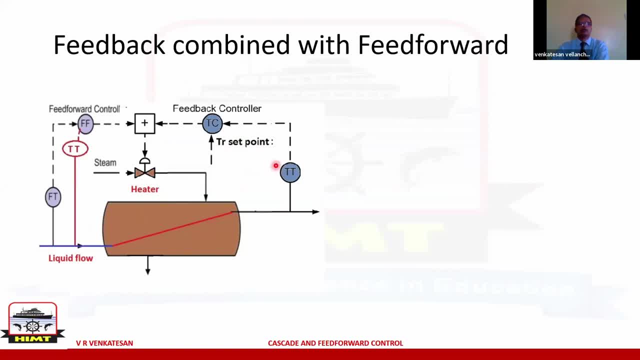 What is this? Temperature? Temperature transmitter. Temperature transmitter is there? Temperature transmitter is telling like this: Now you say: I want 95 degrees, set point here. This is the controller. So this will be your usual P plus I controller. So the output of 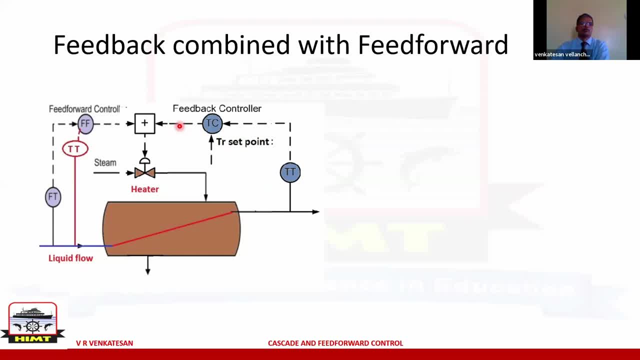 this controller will come. Purifier heater should be PID, So it should be PID, So the output of it comes. These two outputs are combined. This is called as a summing relay or a summing function. Both the outputs will be added. 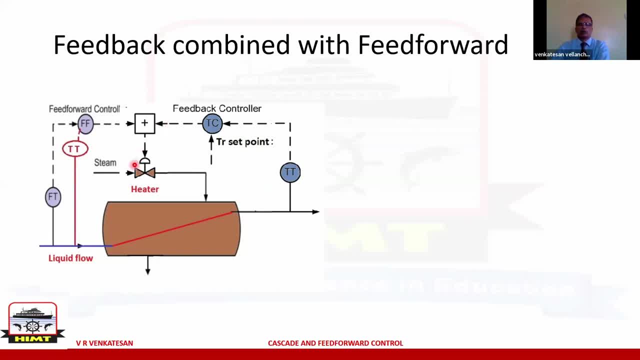 and it goes for the steam heating. So in this case it takes care of both. So if the oil flow changes, definitely it will correct The temperature changes. if the steam pressure changes or the efficiency drops, In that case also it will correct. 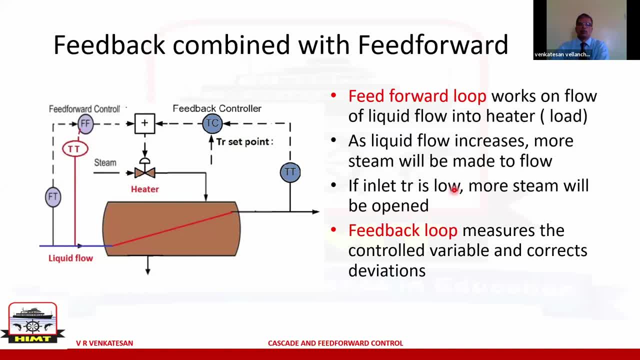 So all this is there. Inlet temperature is low, Most Sorry, Sir. one doubt, sir, In this case of controller, which is the master and which is the slave. sir, This is not master slave, Okay, Master slave is serial. 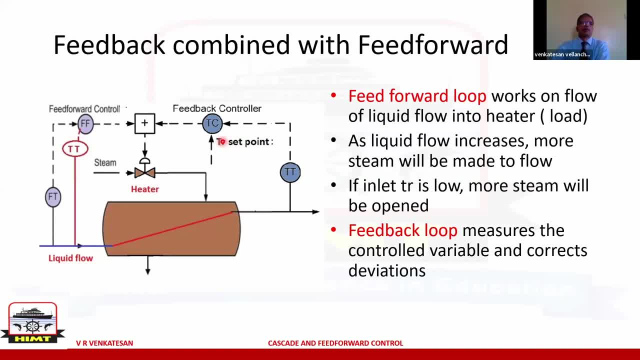 Okay, This is parallel. You can see, this is parallel. The output of this controller goes parallel to output of this one. They are added up Here. there is nothing called master slave, Okay, sir, But there is a question of the main controlling part, That 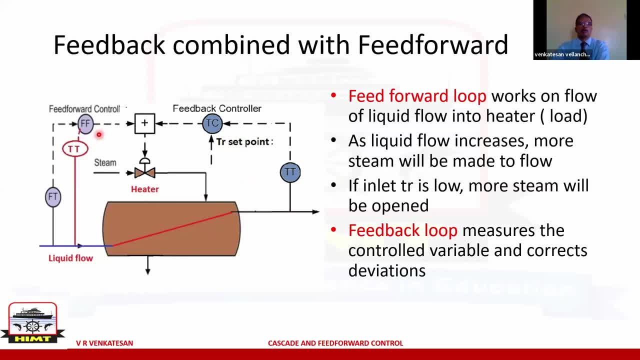 you will see, Both are not equal in their effectiveness. That part you will just see. So if steam pressure falls, will this take care? or if the heater gets fall, will it take care? All of this This control can handle, Sir. It can take. 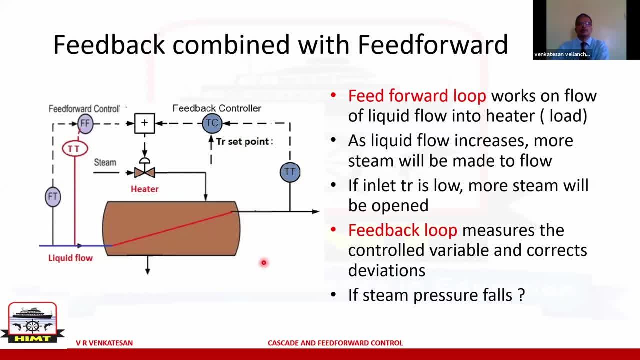 care, Excuse me, We are Venkateshan. We have one question: Definition or difference between feedback and feed forward Comes later We will see, Sir. My name is Venkat. I have a question, sir, A little louder please. 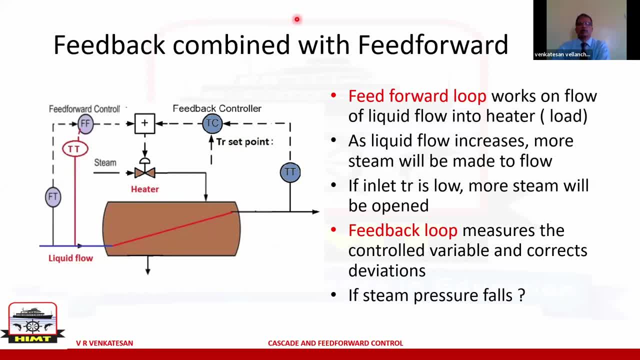 Yeah, Definition. and I have a question, sir. Yeah, Go ahead, Sir. As you have mentioned swell and shrinkage, sir, By using only feed forward type of controller, we can actually tackle the issue, right, sir. Yes, Yes, That is why it is used. 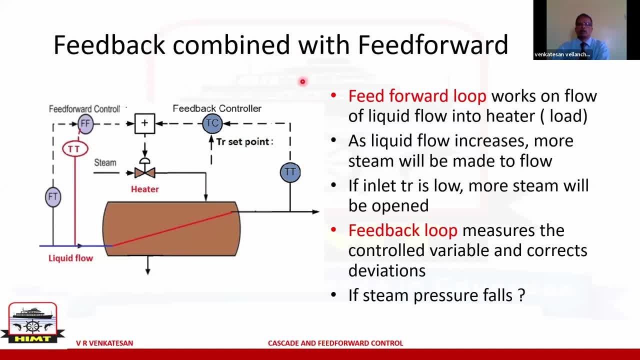 Okay, Okay, sir, Thank you. That is why it is used If you do not use feed forward for water level control. the problem with this swelling business is that in a boiler, what is the temperature of the water? Is it a fixed value or does it change? 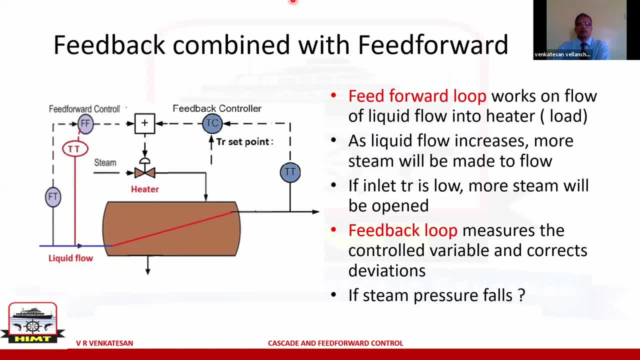 It changes, sir, According to the requirement, it changes Changes. No, No, No Water temperature. Boiling Water is boiling inside a boiler, Right? So if the temperature of the boiler water, is it a fixed value or does it change with pressure? 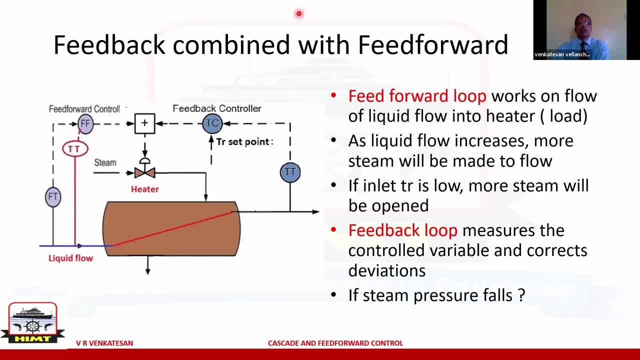 Difference on water pressure. Changes, Changes with pressure, Changes with the pressure, Right. So what is going to happen is imagine that in your boiler pressure is 16 bar. 16 bar steam pressure will correspond to something like 205 centigrade. 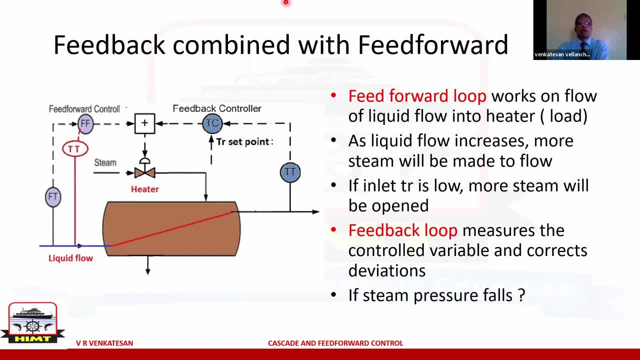 temperature. The water will be at 205 degrees when 16 bar steam is being produced. Now imagine steam demand increases. When the steam demand increases, what will happen to the pressure in the boiler? It will reduce. It will reduce When the pressure. 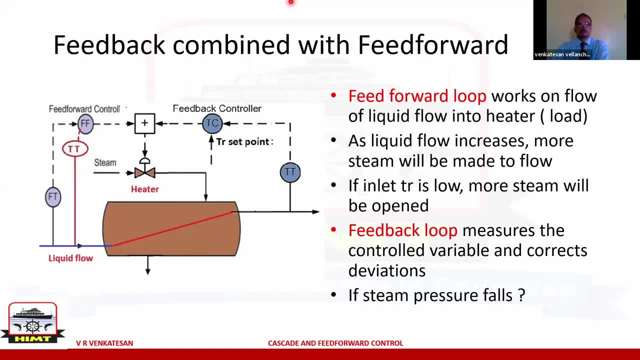 drops to, let us say, 15 bar, the boiling point, or what is called temperature, will also drop. It may be, let us say, 200.. So what is the temperature of the actual water? If steam pressure drops to 15, can the water temperature also drop? 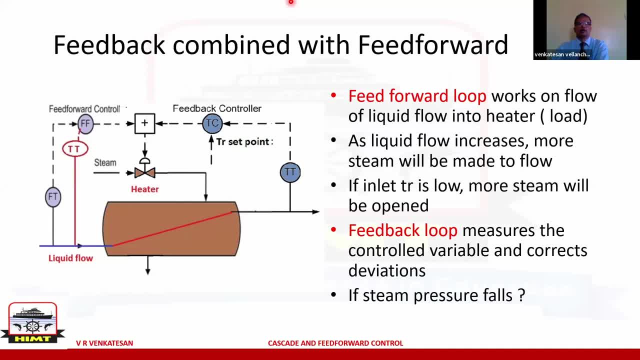 to immediately to 200?? No, sir, It cannot. So the water in the boiler will be at 205 degree centigrade, But the boiling point is lower than that. It is only 200 degree, Right, sir? So what is going to happen inside the boiler? 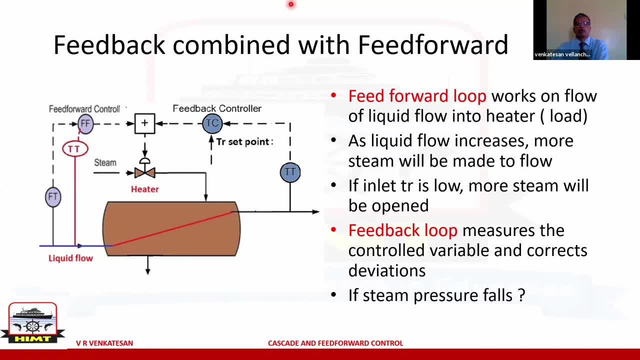 It boils up, The generation of steam becomes very, very rapid. You will get steam bubbles forming. Steam bubbles are forming even otherwise, But the rate of steam generation becomes very high And the steam bubbles form throughout the boiler And steam occupies much more. 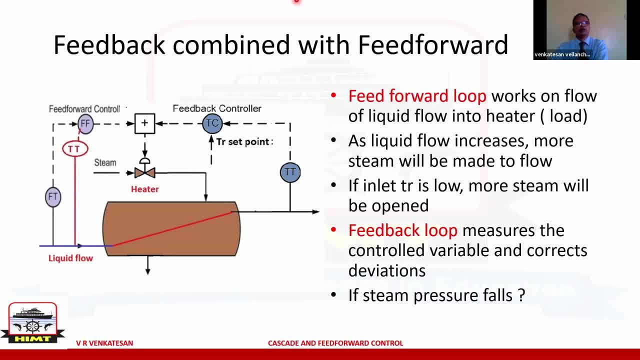 volume than water, Right When water turns into steam. So what is going to happen is the boiler, very large number of steam bubbles will form. Due to this. the water level will rise, The real rise in water level. So why is the water level rising? 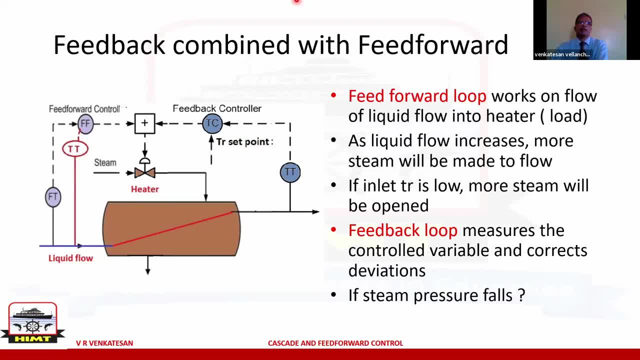 is because steam pressure is dropped suddenly. Why is the steam pressure dropped suddenly? Because demand increased suddenly. So if I have only error based control- Error based control- What will the controller do then? Water level is rising. What will the controller do? 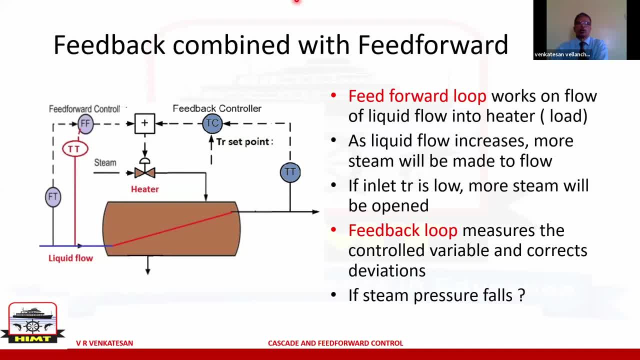 It will stop reducing the level, It will close the feed, It will stop the flow, It will start reducing the feed water. But what is required? Steam demand is increasing. So what is required now? Water is required. Actually give more water. 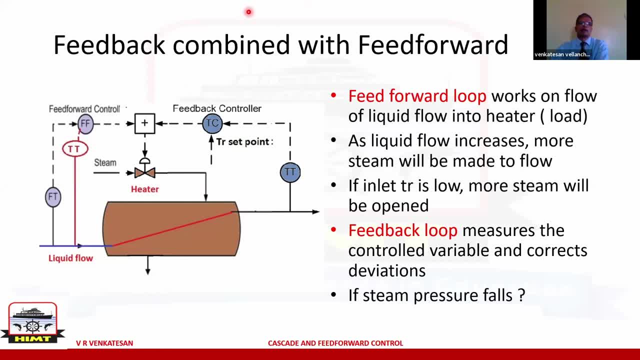 That is the reason. So, especially in a boiler feed water, this feed forward control is also used along with this. So steam demand is also measured And water level is also measured. Okay, That is what you call as two element water level control. 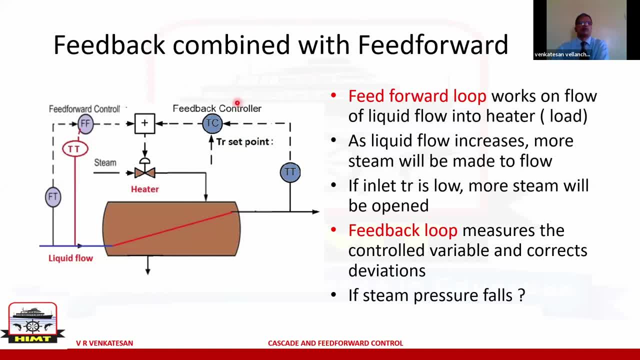 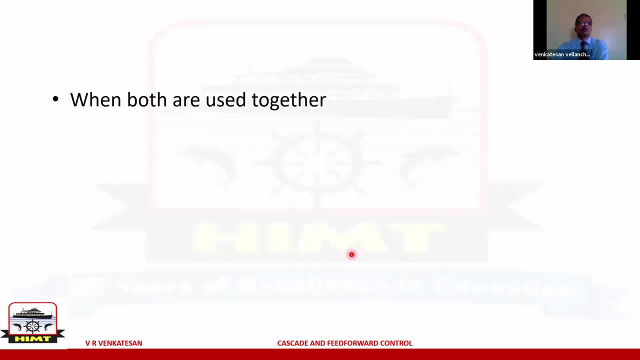 Okay, Coming back to this point, So you can see this part is feed forward and this part is feed back, And the combination of this it will be possible to control much more effectively. So when both are used together, the feed forward will do the main. 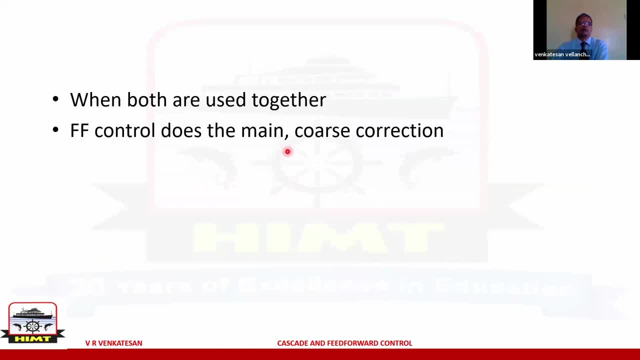 controlling, But its control will be coarse. Coarse means it will not be exact. As soon as the steam demand increases, feed water will increase. Or as soon as the steam demand increases, firing rate will increase. But the feed back control will give the. 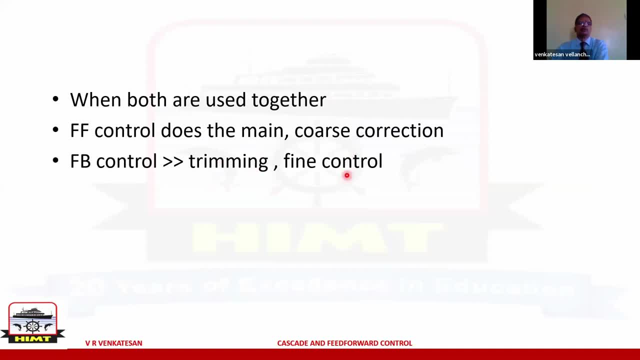 exact value, How to maintain If you want 16 bar. finally, 16 bar will come because of the feed back control. So this is the comparison. When you use together, the first reaction always comes from feed forward part And it will do the bulk of the correction. 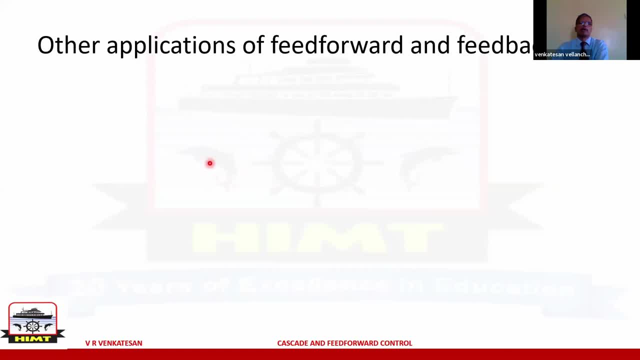 But the fine adjustment is done by feed back. There are other examples of feed forward and feed back control, combined control. One is AVR. The purpose of AVR is to maintain terminal voltage when the load is changing Correct. Now normal feedback control means. 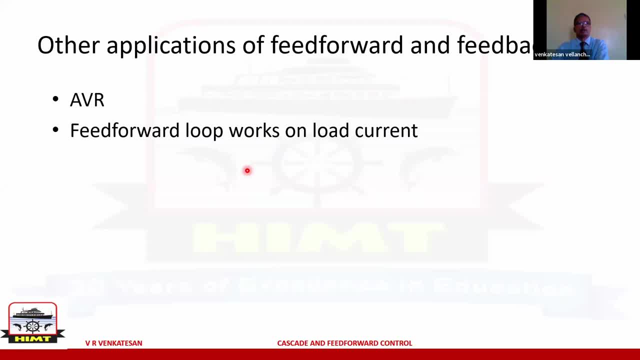 you measure the terminal voltage and when the terminal voltage reduces you can increase the field current. But feed forward loop means you look at the load current. Why should terminal voltage drop In an alternator If the load increases? When the load increases, load current increases. 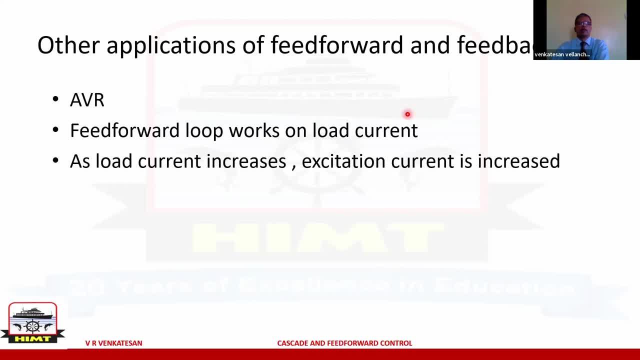 There are many reasons you would have studied. There is armature reaction. There is voltage drop inside the armature, There is governor's droop. because of it the rpm drops. So for all these reasons, terminal voltage will reduce. So if AVR measures the terminal voltage, 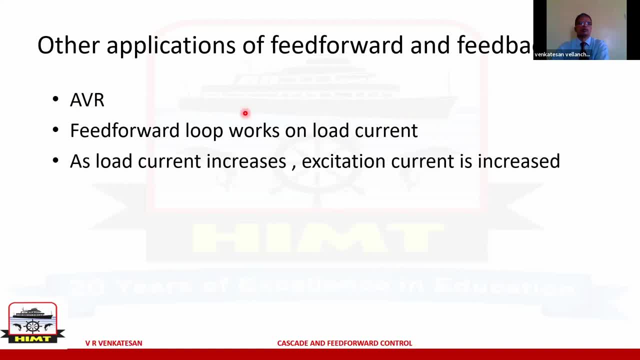 and then it corrects. that is called feed back control. Feed forward means you measure the load current. So as soon as the load current starts increasing you can increase the excitation current. And feed back loop works on the terminal voltage So you can have 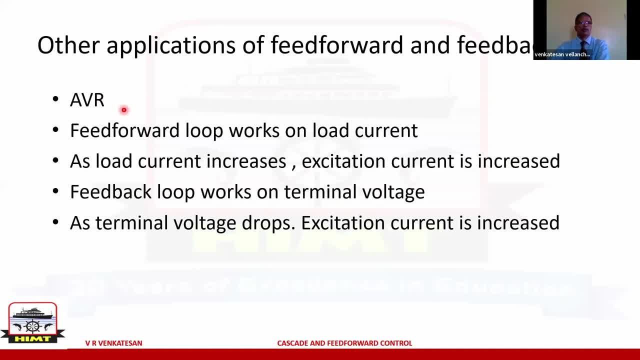 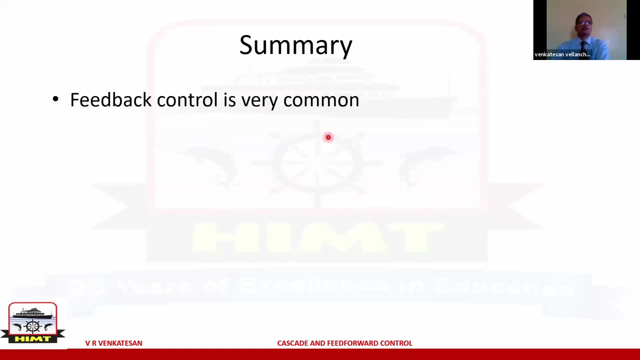 AVR which is only error based or which is error and load based. Definitely the combination will be faster. So to summarize, these are the few things. Feed back control is very common. Feed back control is always error based. That means deviation will take place and then will be corrected.